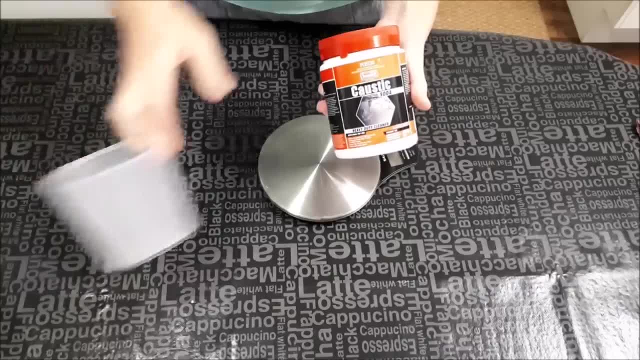 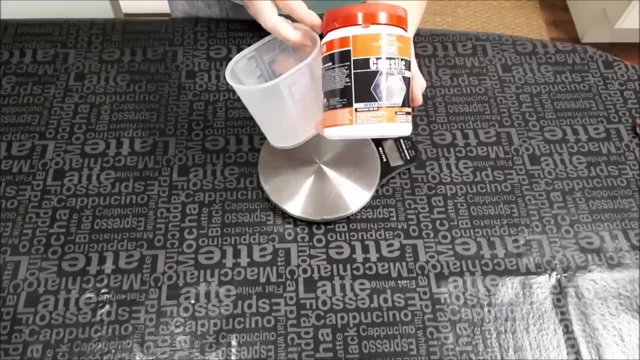 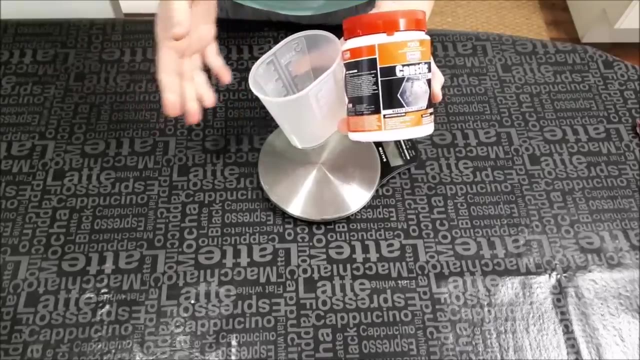 your caustic soda with your water. it generates a lot of heat and the solution is quite hot to begin with. Now, ideally, in this soap making method, which is called cold process soap making, all of the ingredients are cool or at room temperature before you start. That just helps to keep the process nice. 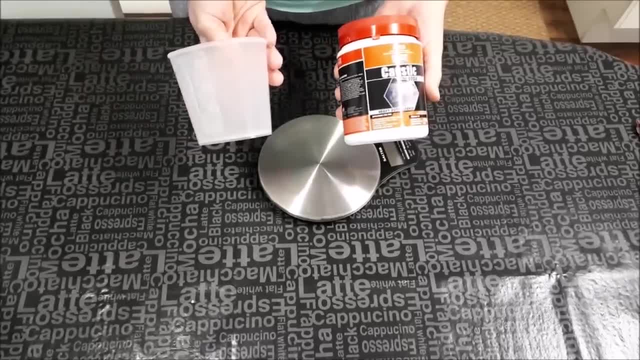 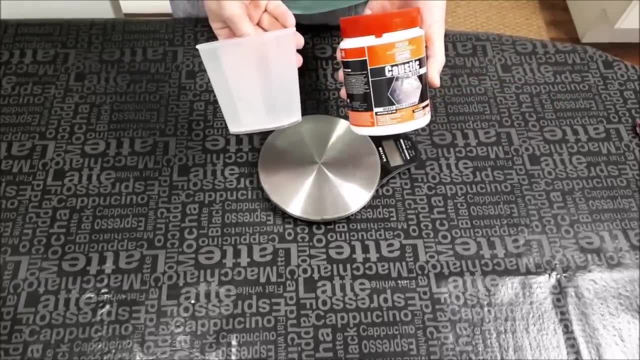 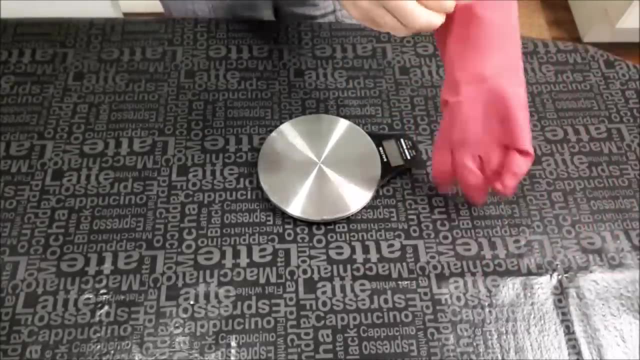 and slow when you're making the soap, which which makes it easier to handle. So I do this first and then set this aside and let it cool almost completely before I make my soap, So to make your lye solution. this is probably the most dangerous part of soap making. Put your gloves on and you need. 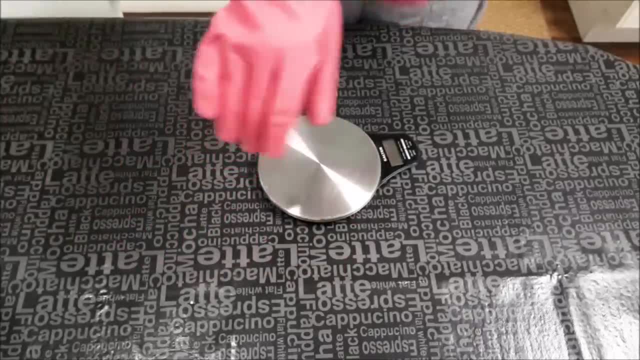 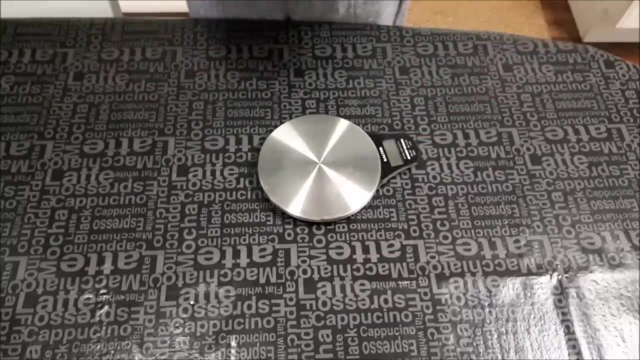 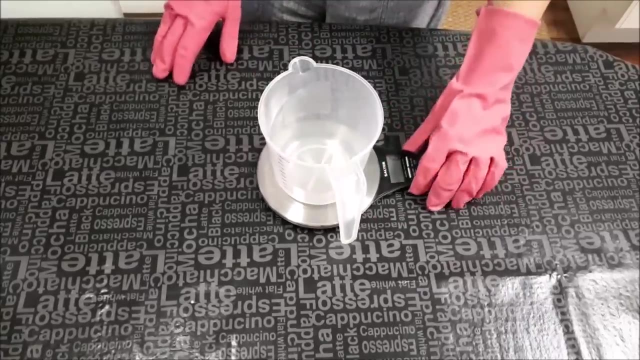 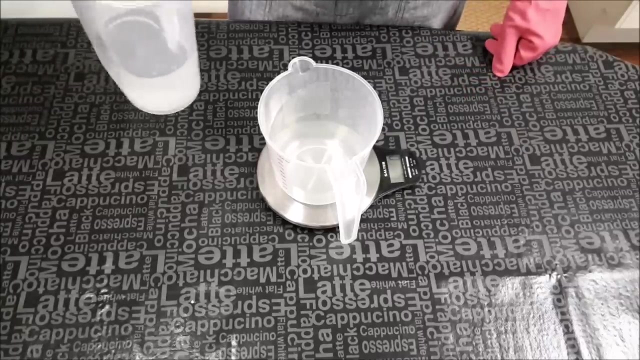 your digital scale for this as well, Your safety glasses and, first of all, going to weigh out the water. So in this recipe I'm using a 40% lye concentration solution. So that is a hundred and ninety nine grams of water. So I'm just pouring. 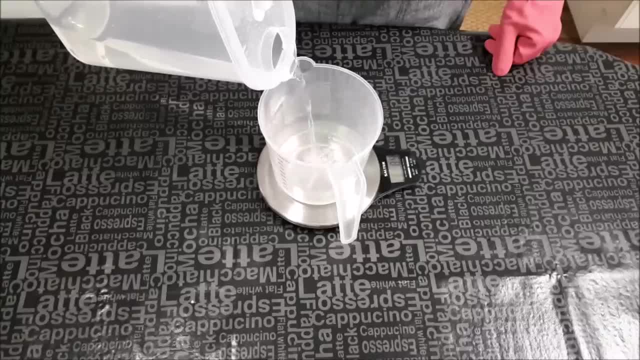 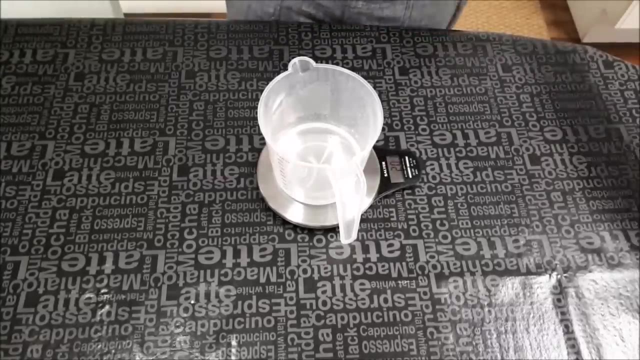 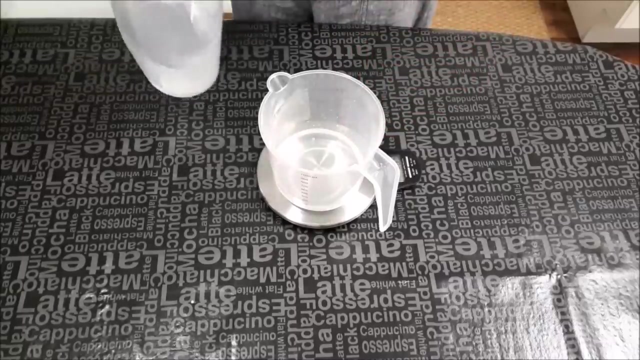 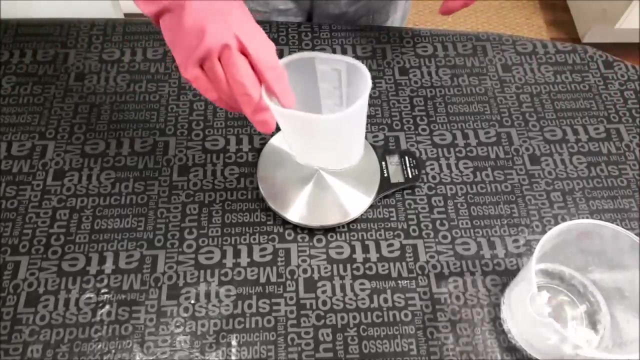 that out. Sorry, this is a bit of a slow, boring part, but I'd really like to show you the the full process. I've got a little bit more in there than I need. Sometimes I get a little bit more. There we go 199.. Okay, so the water is weighed. Now I weigh my sodium hydroxide separately. 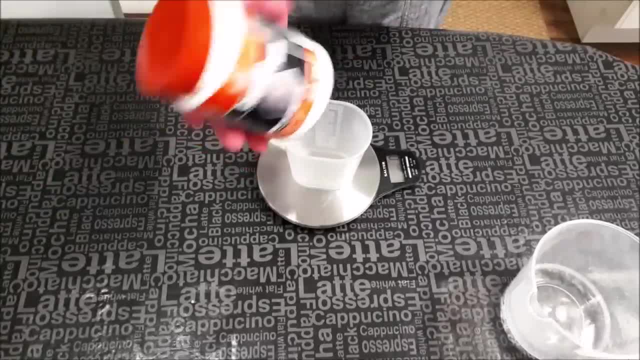 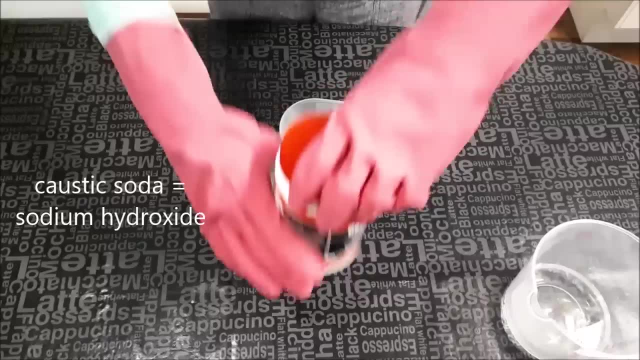 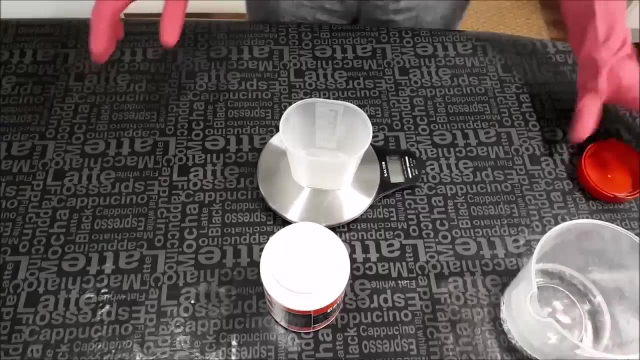 which is pretty important. Just shake your jar of caustic soda or sodium hydroxide. Just give it a shake, because sometimes it can form little lumps in there which makes it a bit harder to work with. So you open your container and then I like to just spoon it in with a spoon. Sometimes you 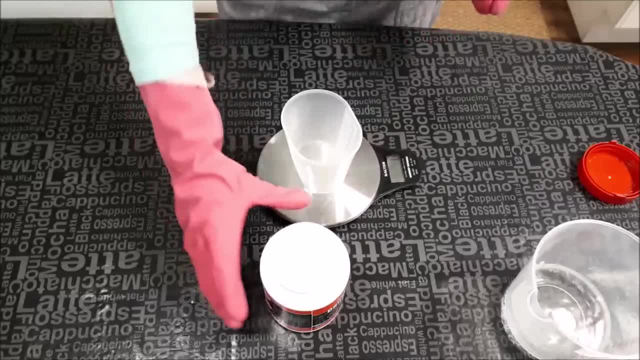 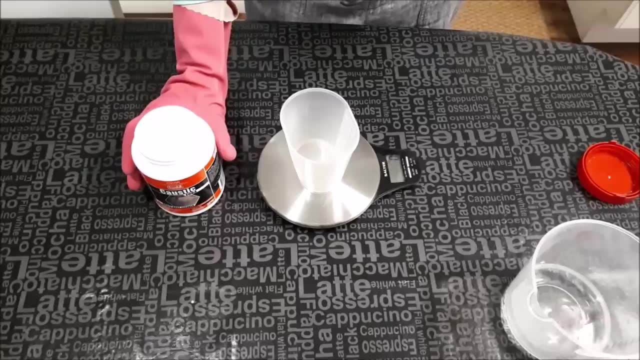 get your caustic soda. it comes in big jugs that you can kind of pour it out of, So just use what's the safest for you. So in this recipe I need a hundred and thirty three grams of caustic soda, So I'm going to spoon that in, Make sure. 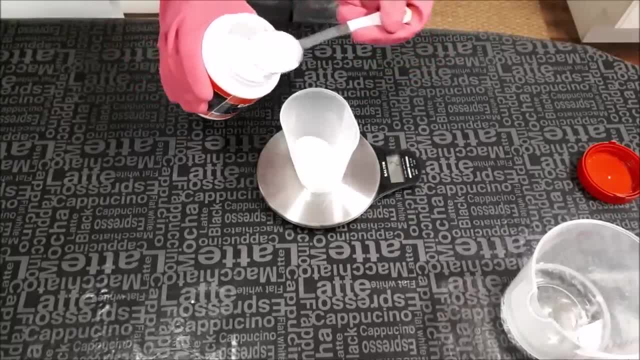 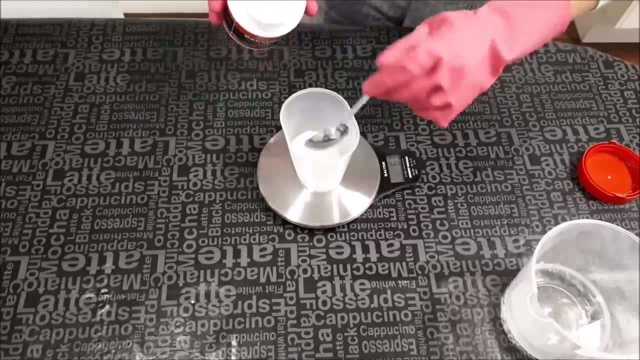 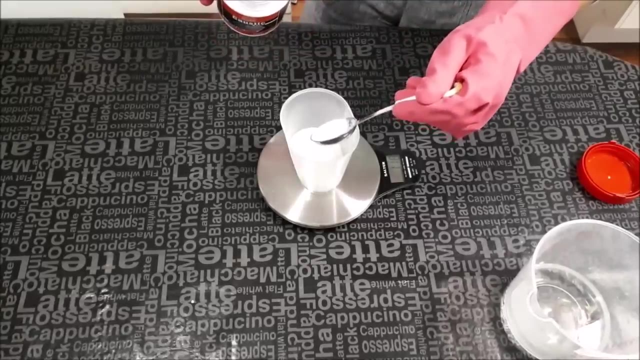 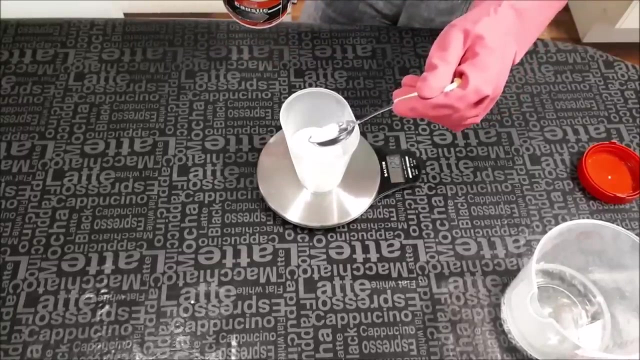 you zero out your scale before you go Doing it. this way is really good, because if you get a bit too much, you can just put it back in. So it's easy. You're not going to make any mistakes this way. 130.. 132.. 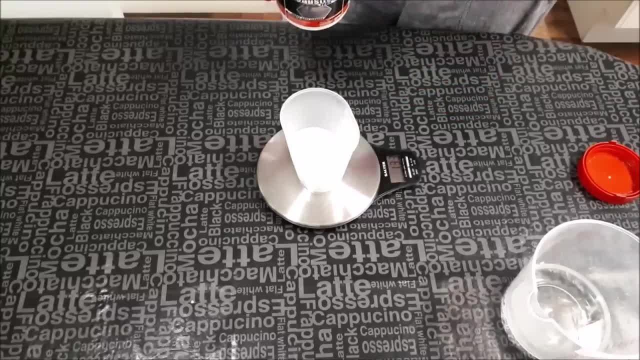 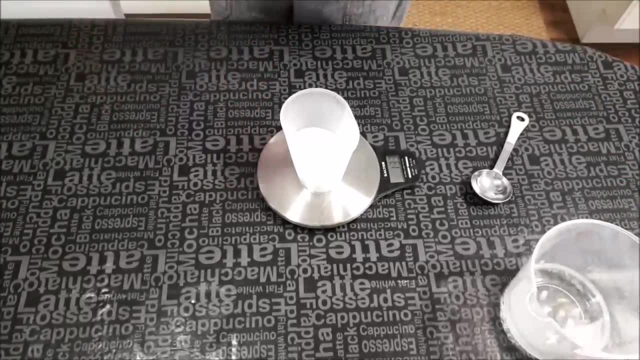 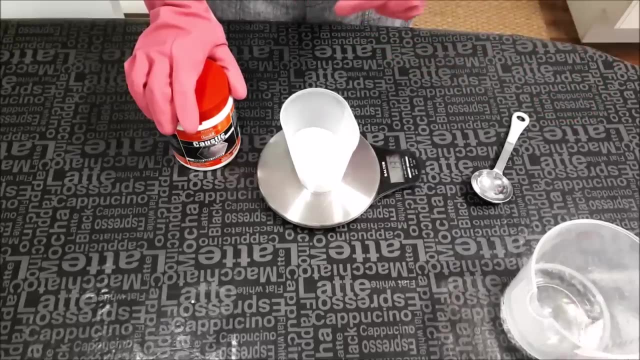 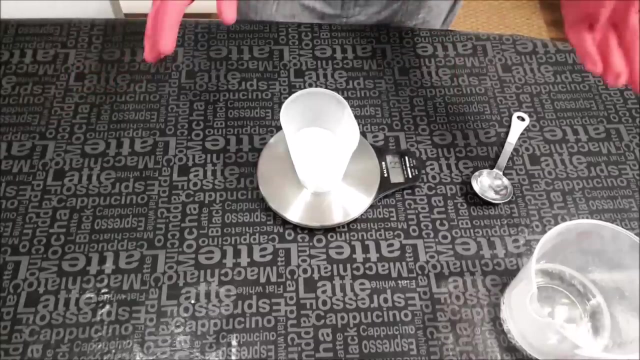 It's important that you get these measurements really accurate because, as I said in my other video, each oil has its own particular fatty acid profile, which has a different saponification value. so different oils require different amounts of caustic soda. So please don't substitute oils in this recipe, just follow this recipe as it is. 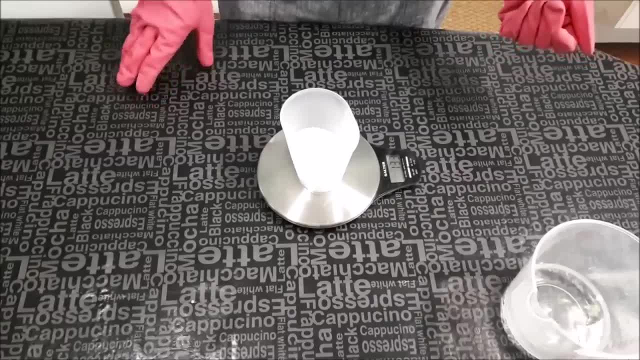 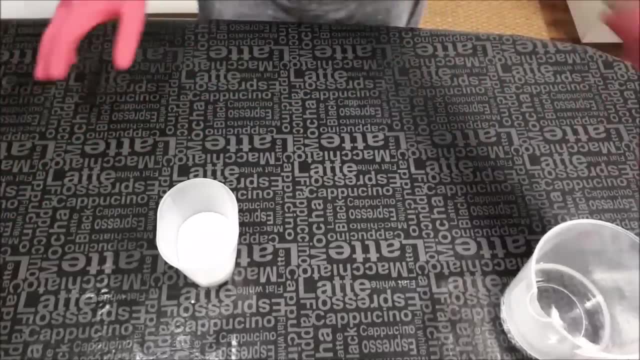 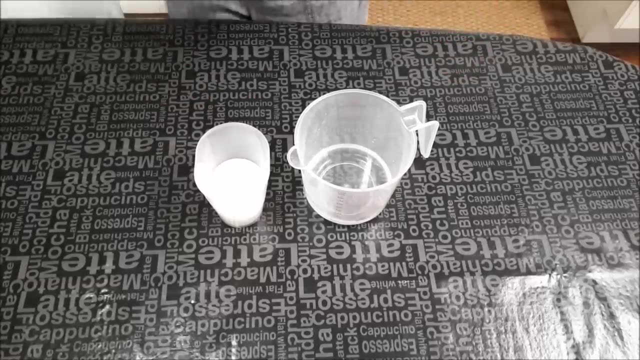 If you'd like to use other types of oils in your soap making, then the recipe would need to be recalculated. Alright, so I've got my 199 grams of water and my 133 grams of sodium hydroxide. I'm going to get my little bendy spoon. 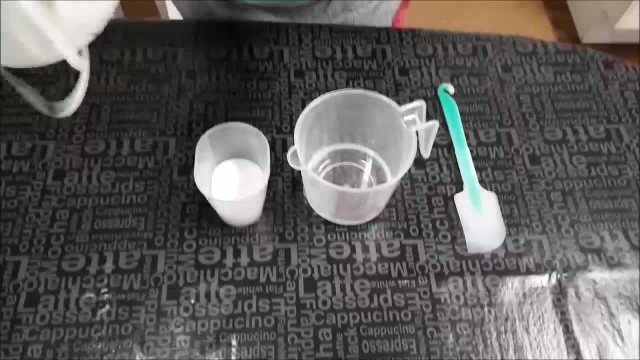 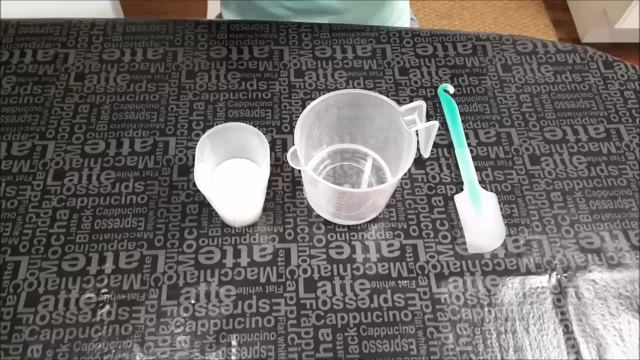 I'm actually going to put my little mask on as well and I'm going to sit down just because, uh, sometimes you do get a little bit of fumes. well, you do get fumes off this and I prefer not to breathe it in. 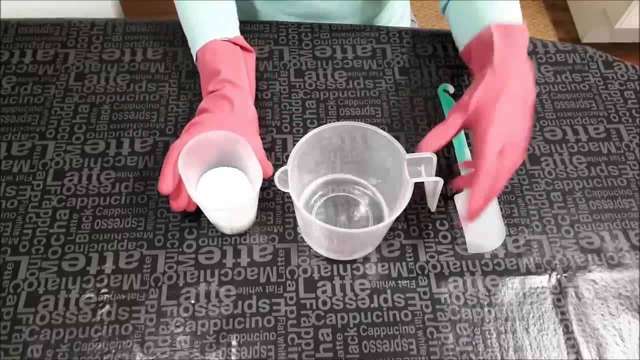 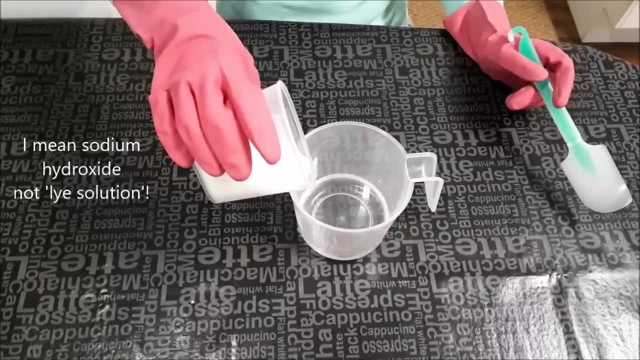 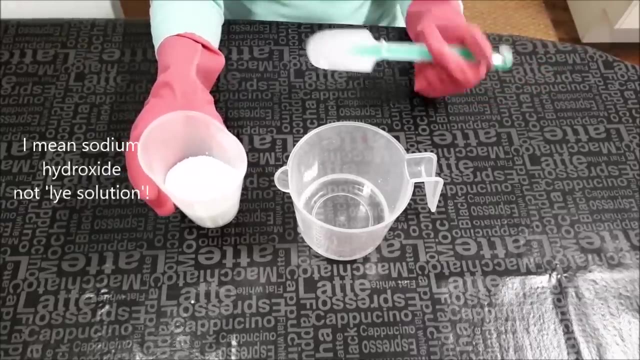 So I've just got my little mask on and then I hope you can hear me- and then you just slowly pour your lye solution into the water. You always, always, always pour the lye solution into the water and never the other way around. 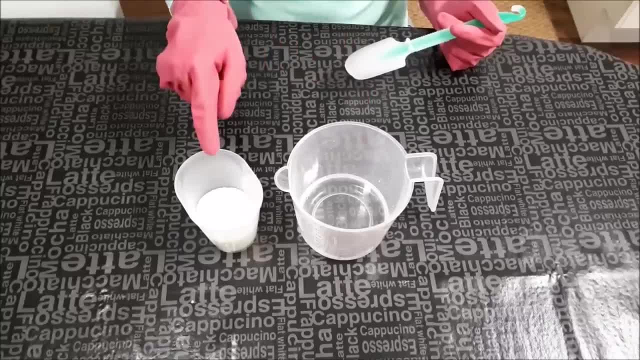 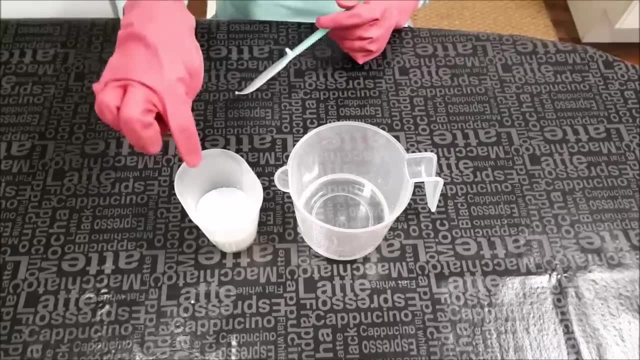 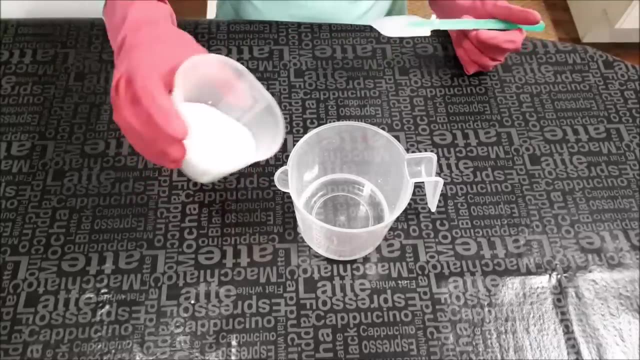 If you pour the, if you pour the water into that, um, it will bubble, It will hiss and spit and carry on, which you really don't want. so you always pour the sodium hydroxide into the water. Alright, here we go. 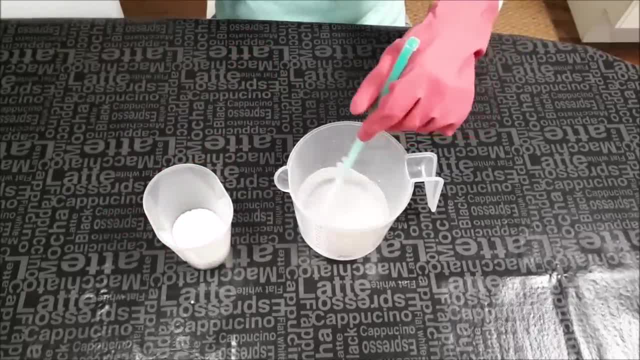 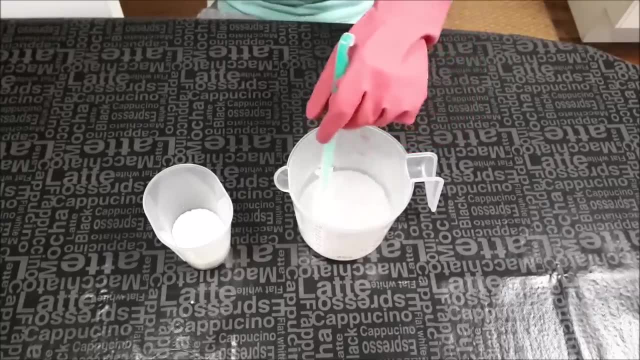 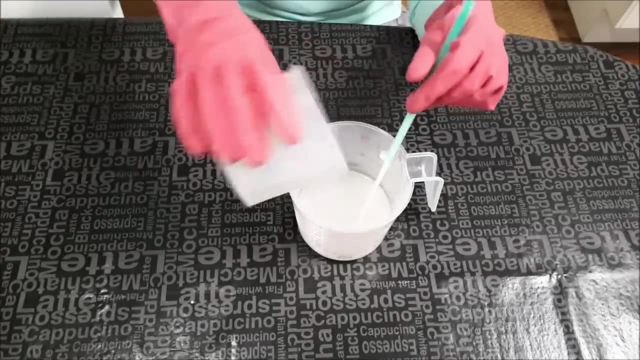 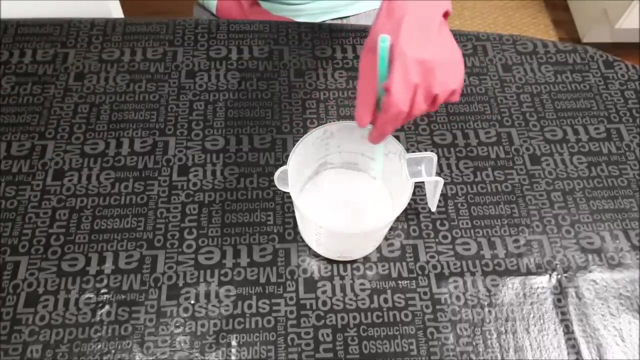 I usually do about half, give it a stir And then put the other half in. Give it a stir. Okay, Give the container a bit of a tap, Pretty much all out, that'll do, And just stir it. It doesn't take long to dissolve. 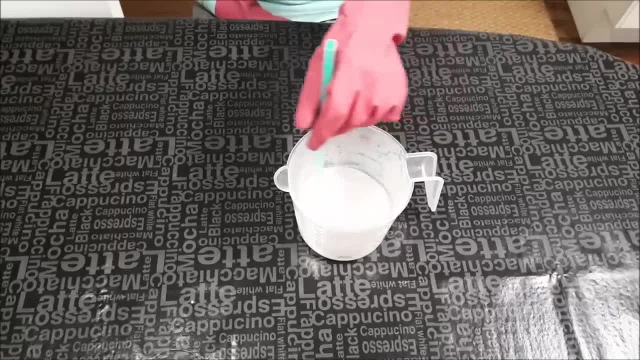 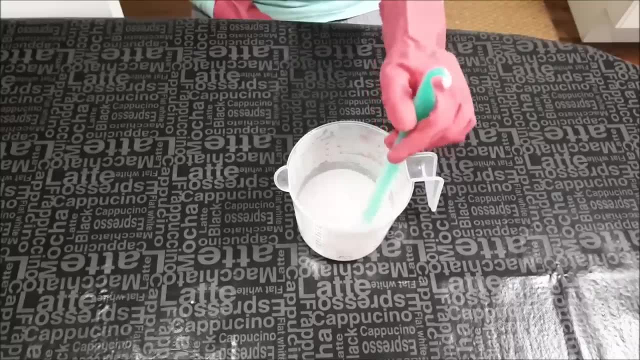 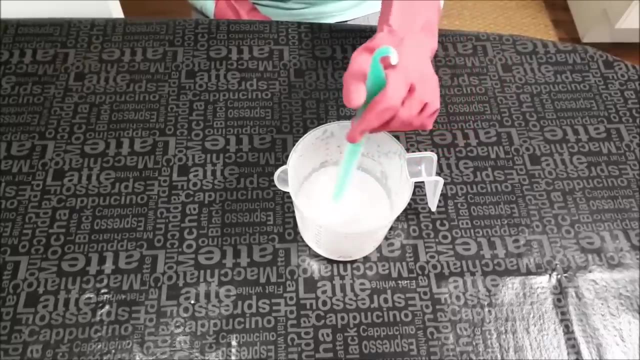 I can see the gas coming off that. um. it will eventually um change from being that opaque colour to being a clear liquid once it's cooled. Um, this spatula goes quite bendy in this hot solution, but it's still okay, so 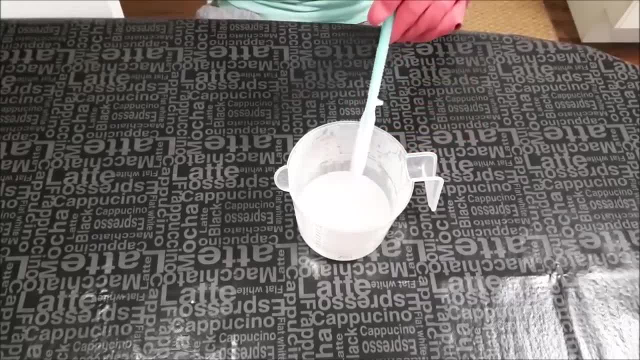 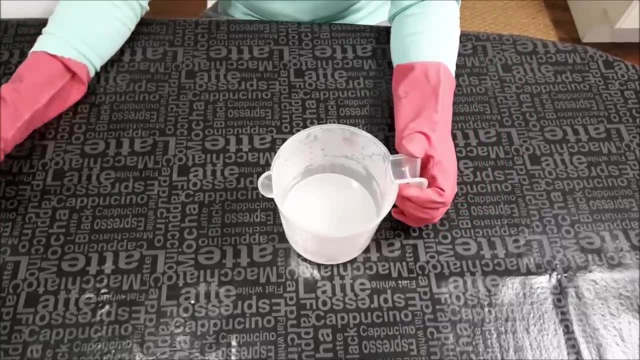 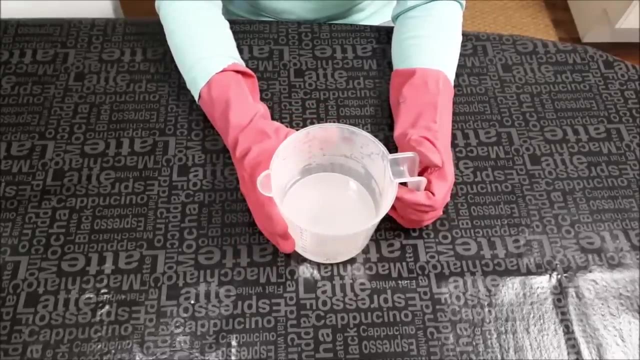 There we go. That's enough stirring, That's all you need. Only takes maybe 20 seconds or so, And there is your lye solution mixed. So I will generally put this aside, uh, somewhere very, very safe until it cools off. 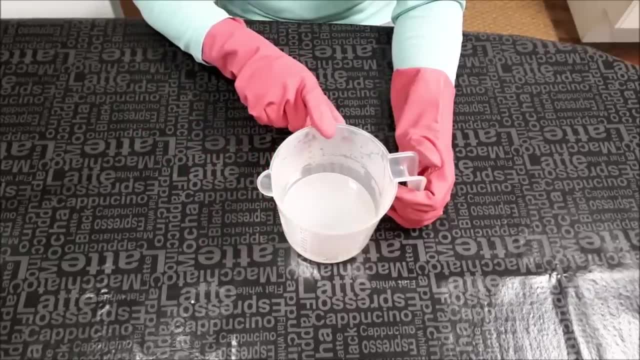 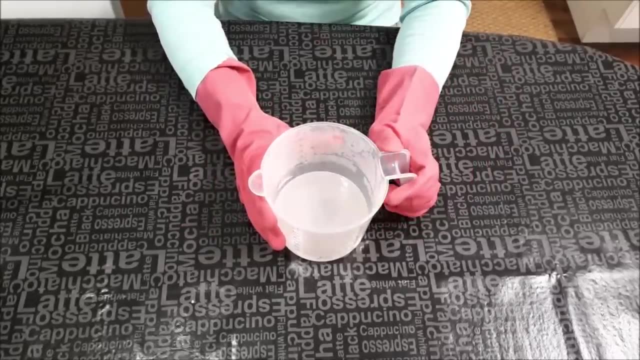 And then if I'm making, sometimes I mix this the day before and then I make the soap um the next day. once this is fully cooled, I will, once this is cooled off, I'll pour this into a jar and screw the lid on the top. 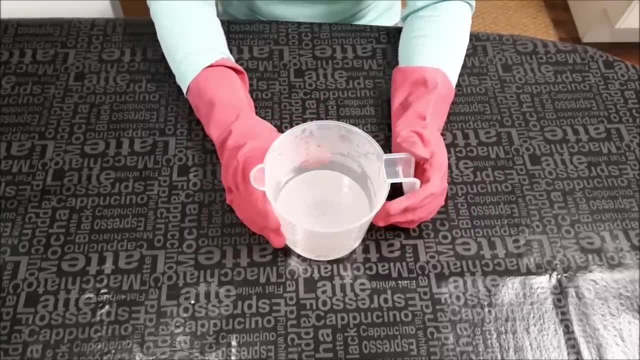 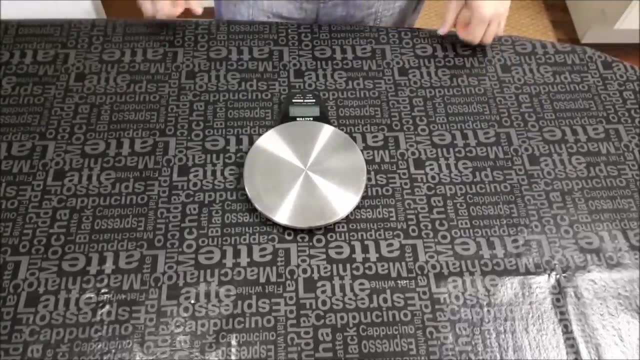 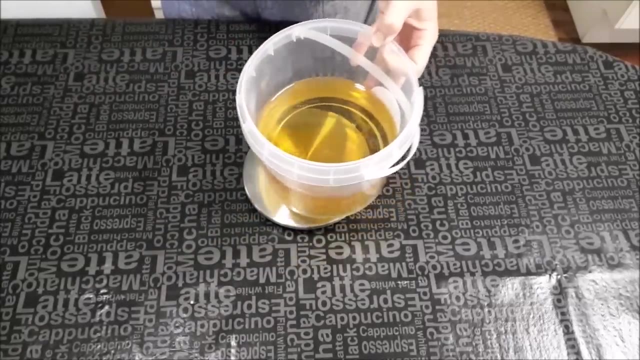 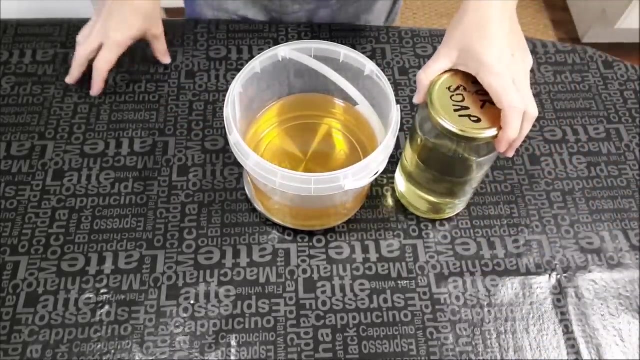 Just to make it a bit safer for storage. Okay, So there's the lye solution. Um, the next step in the process is to weigh out your oils. So I've already weighed my olive oil, just to save time. So in this recipe I'm using 950 grams of olive oil and 50 grams of coconut oil. 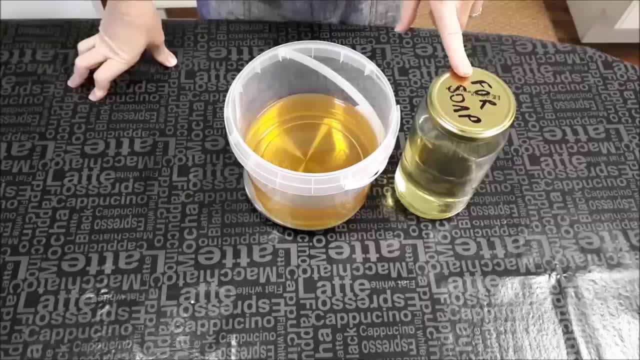 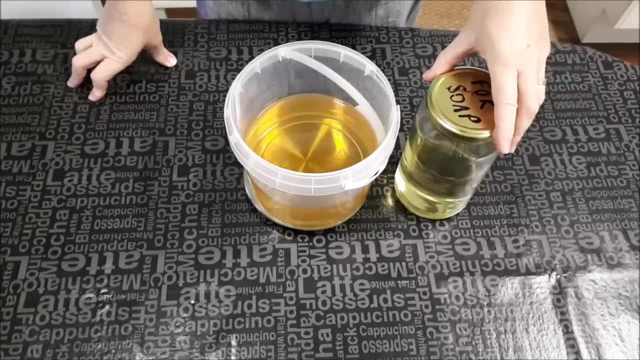 So that will be 95% olive oil and 5% coconut oil. Coconut oil can be very drying to the skin if it's used in a large amount in a soap recipe. Um, so the bulk of this is olive oil, All right. 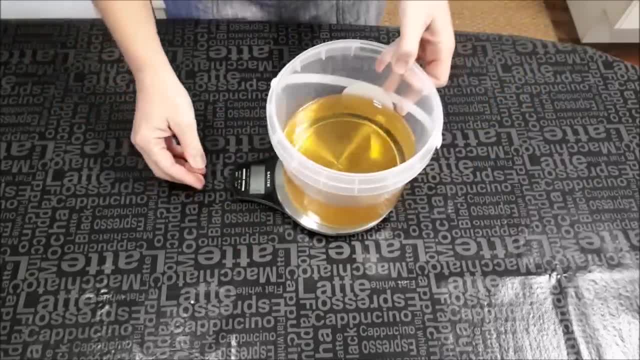 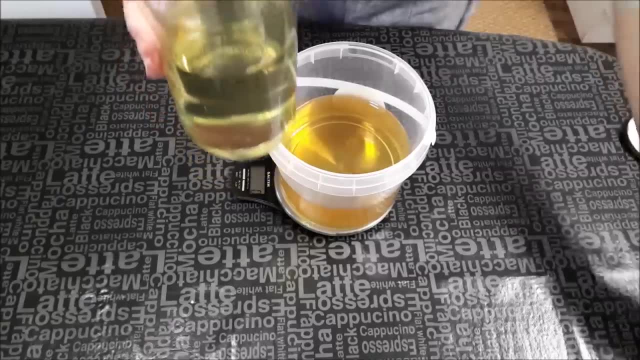 So I've got my 950 grams of olive oil already in there. I'm just going to zero out my scale. I've just melted this coconut oil in the microwave for a little while, but if you've got a sunny day, you can just leave it out in the sun for a while. 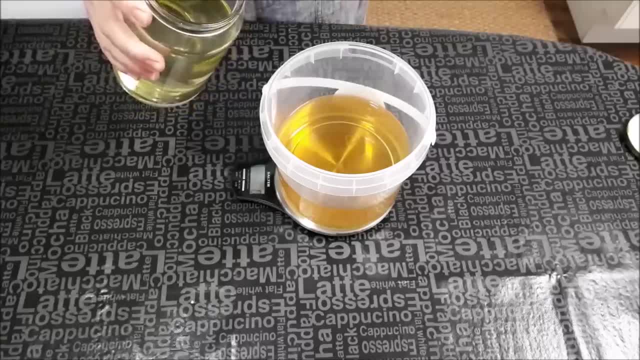 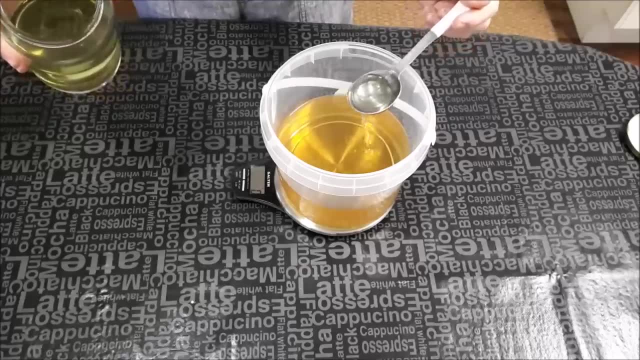 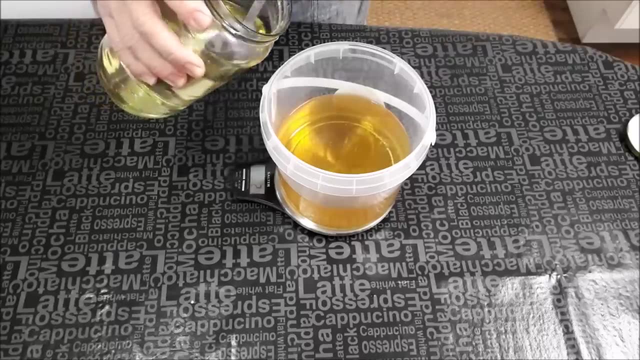 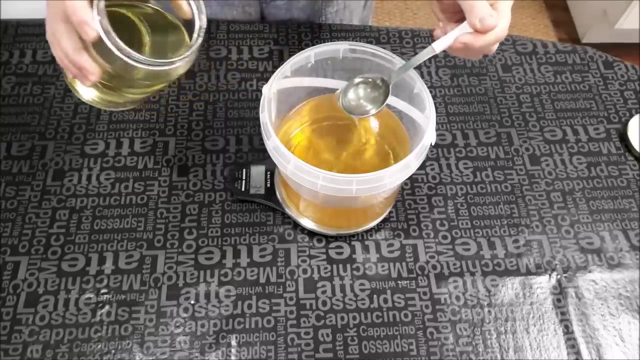 Unfortunately, It's a sunny day today. um, because this is only 50 grams going in here, I'm just going to spoon it in just so that I don't make a mess and um make make a mistake. So that's 10, 21,, 34,, 47,, 48,, 49,, 50,, 51,, 52,, 53,, 54,, 55,, 56,, 57,, 58,, 59,, 60,, 61,, 62,, 63,. 50,, 52,, 53,, 54,, 55,, 56,, 59,, 60,, 62,, 63,, 65,, 65,, 67,, 68,, 87,, 88,, 89,, 90,, 90,, 91,, 92,, 93,. 95,, 91,, 92,, 93,, 95,, 96,, 97,, 98,, 90,, 91,, 92,, 93,, 92,, 93,, 94,, 94,, 94,, 95,, 95,, 96,, 96,, 99,. 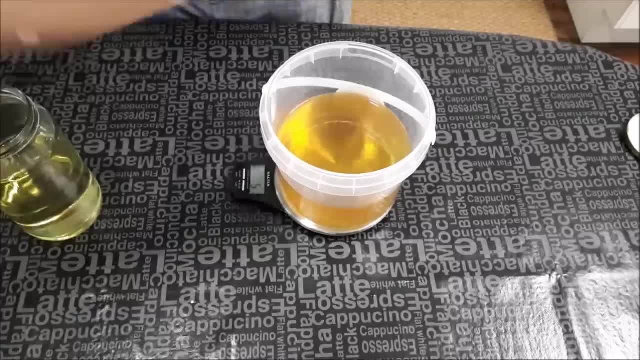 95, 100, 100, 100,, 100,, 100, 100.. There we go, Oh, 51.. That's okay, All right. So there's my oils done, So my olive oil and my coconut oil ready to go. 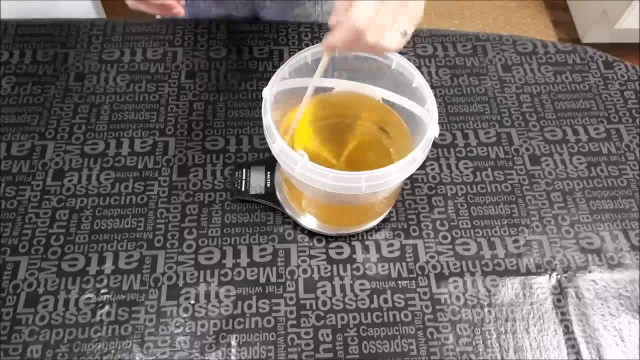 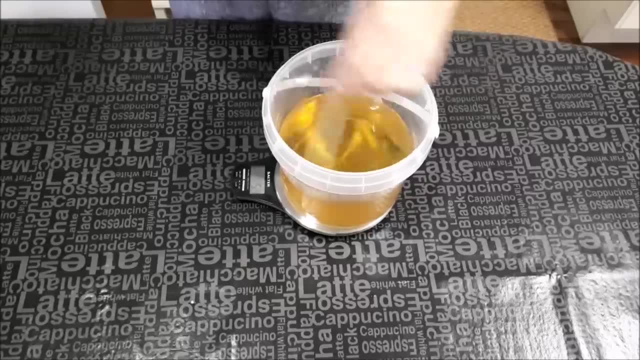 I'll just give those a bit of a mix together. Just have this chopstick sitting here, Um, just mix those, and then I'll go and get my colors and things and I'll mix them in and then we'll be very soon, uh, making the soap. 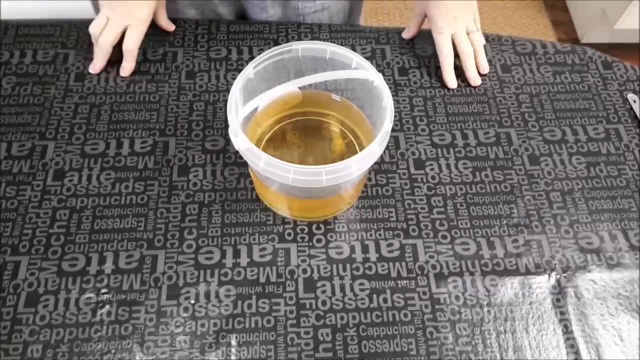 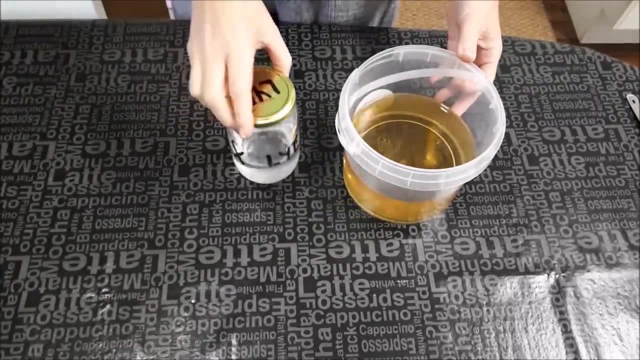 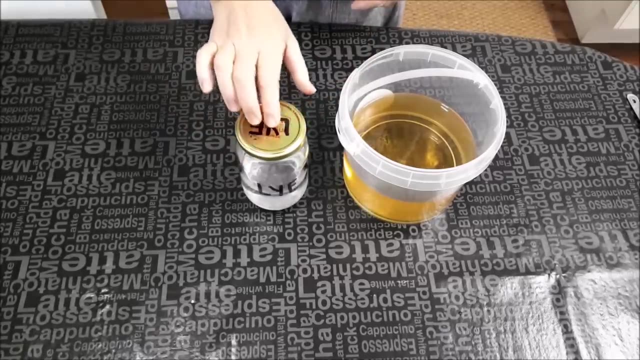 okay, so everything is ready. now I'm ready to make the soap, so I've got my oils. I have a I lie solution, sodium hydroxide solution that I made yesterday, so it's very, very cool. that's identical to the one I mixed before. I've also got some essential oils weighed out. this is lavender oil. 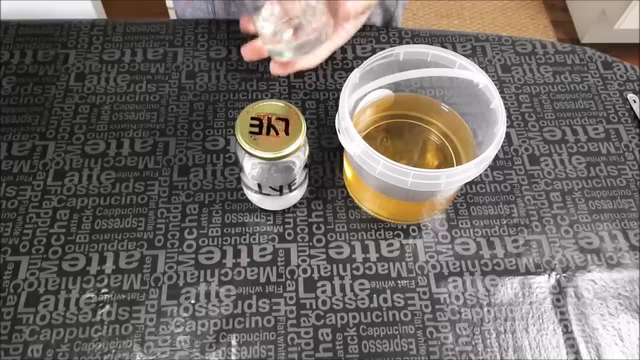 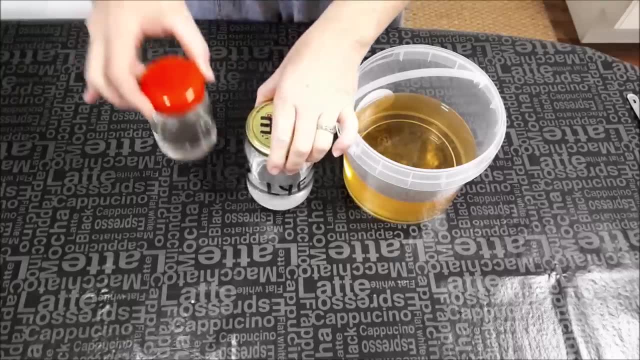 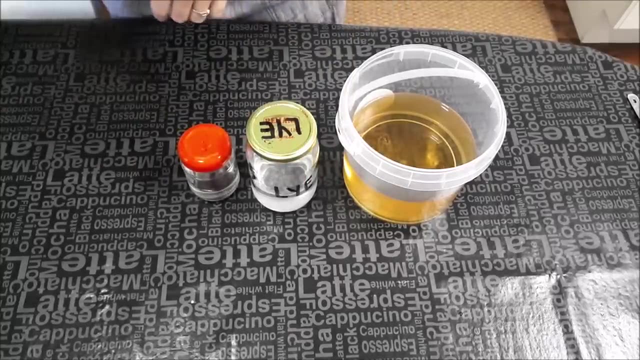 so I'm going to make lavender soap. you don't need to add this to your soap, but if you'd like it to have a nice scent, then I recommend essential oils. just look at online suppliers. that's the best value, and I'm also going to add a few, just little bits to color the soap as well. I should add to: 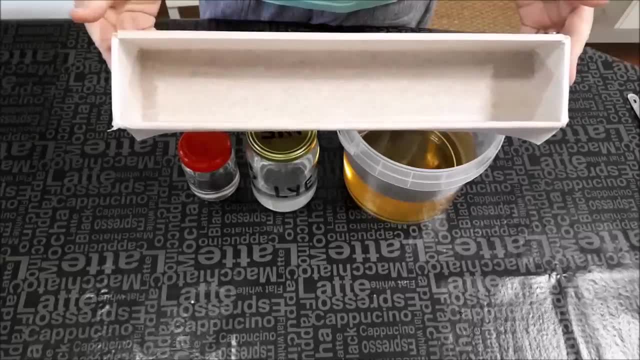 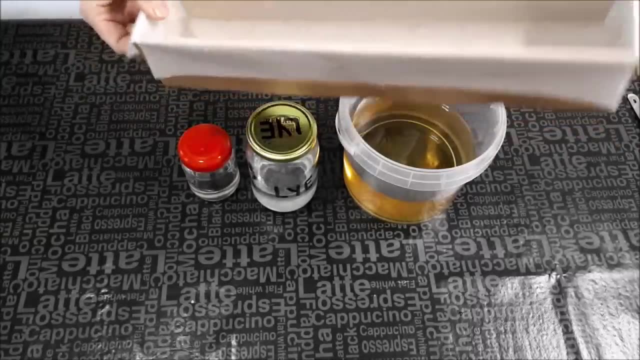 I've also got a mold lined and ready to go. you can use a silicon mold if you want to. it doesn't require any liner, but I'm using this little log mold, so I've got that ready. I've also got a plate and my stick blender ready, so I just 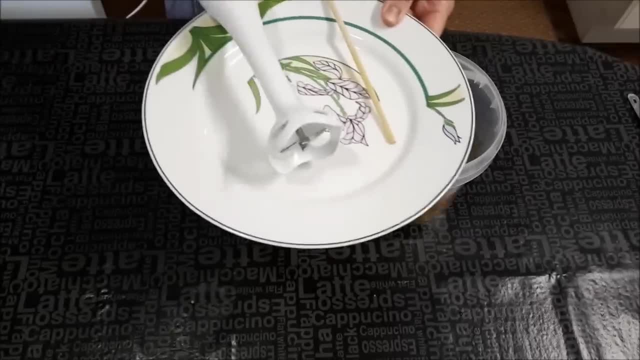 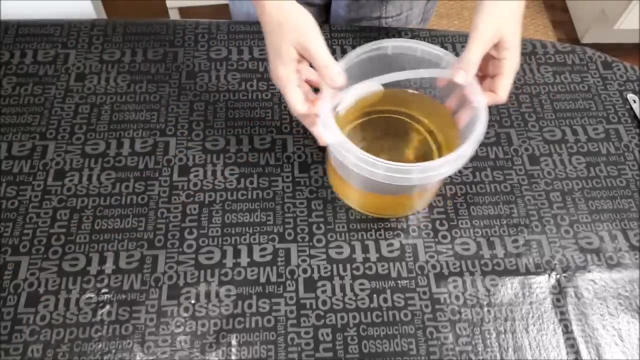 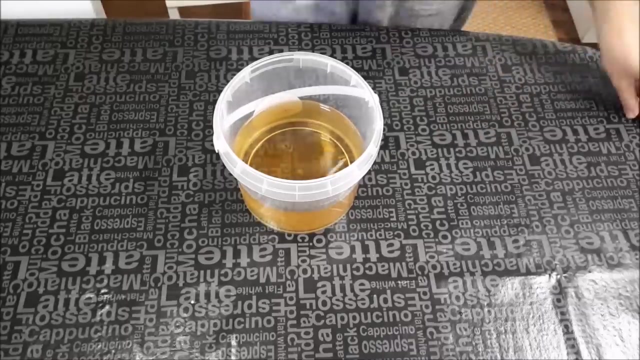 rest this on here and any dirty spoons or anything. they all just sit on the plate. so that's all ready to go. before I put my gloves on and do the- you know, make the soap, I'm just going to put in some of these botanical ingredients. I've just got some lavender powder. that is a funny gray color, but it 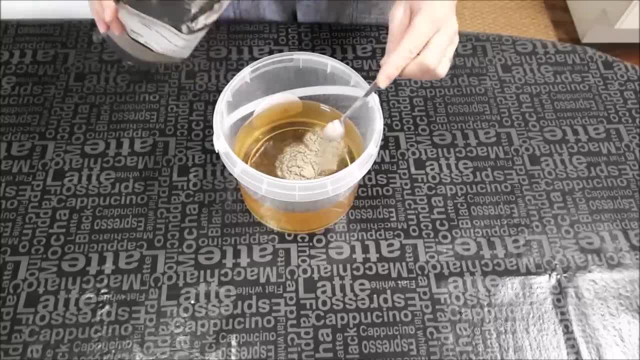 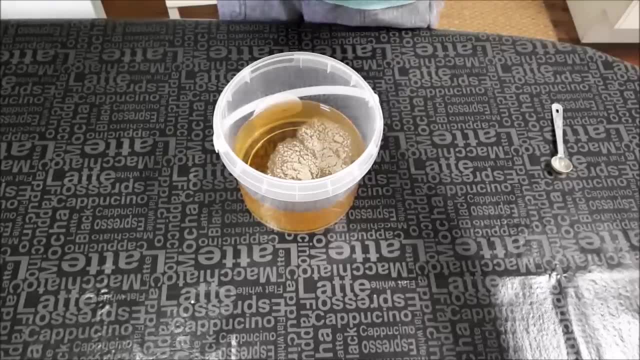 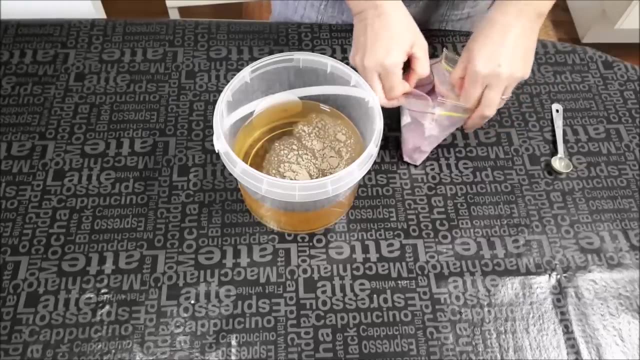 just sort of adds a little bit of texture to the soap. I guess you don't have to add anything to it if you leave it plain. it will just be a lovely white color. I've got a little bit of pink coloring. these are just the um the colors that I normally add to my lavender soap. so just a little bit of. 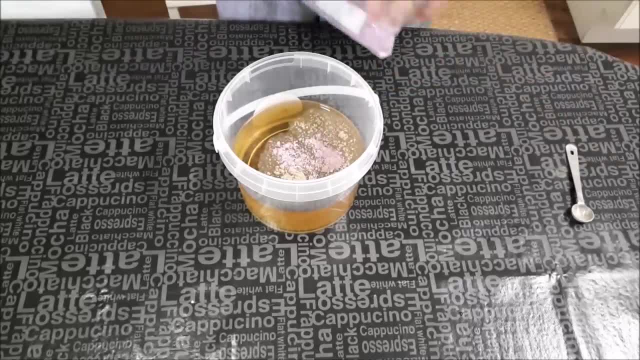 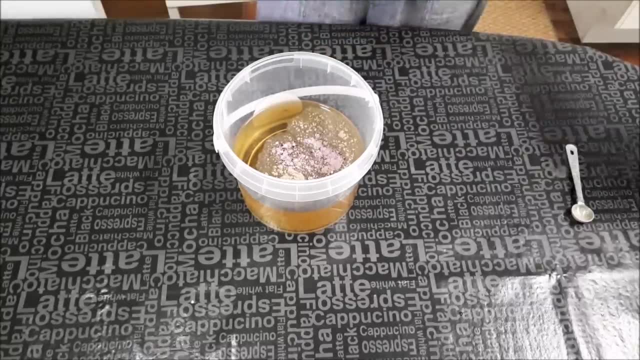 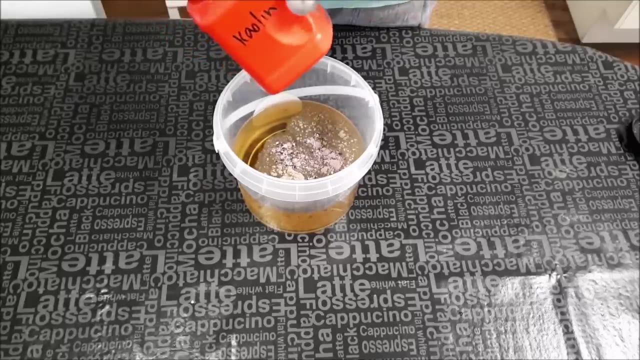 that one. the reason why I'm adding these at the beginning is because I can just stick them, stick, blend them all into the oils. um, some people add their colors in the end, but I like to add them in the beginning. this is um kale and clay, white kale and clay, which. 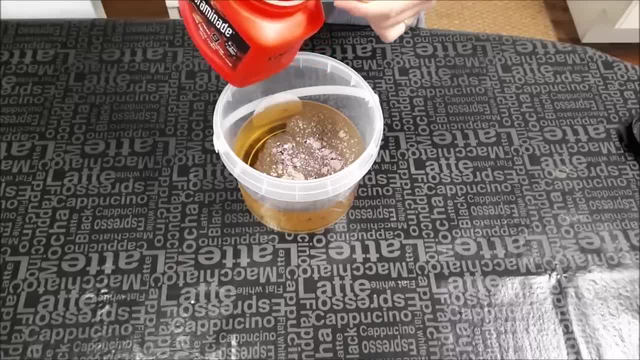 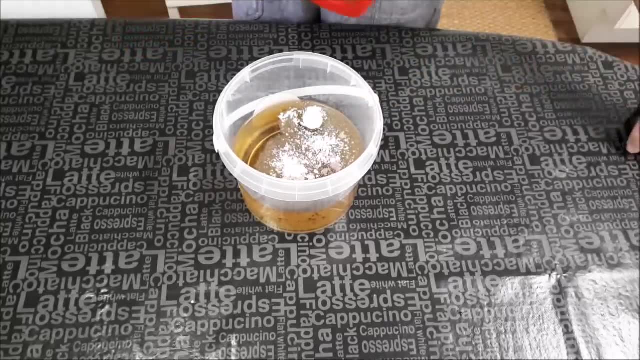 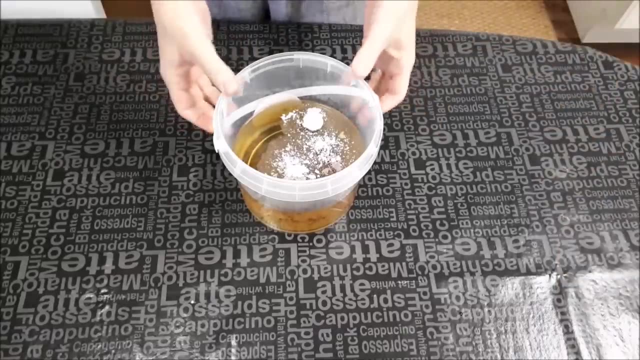 is in a lot of face masks. it's a lovely Australian white clay that will kind of just add a little extra quality to the soap, I guess, but this is totally optional, um, so yeah, you can add all this stuff at the end, which at that stage it is easier to see the color because the soap is emulsified. 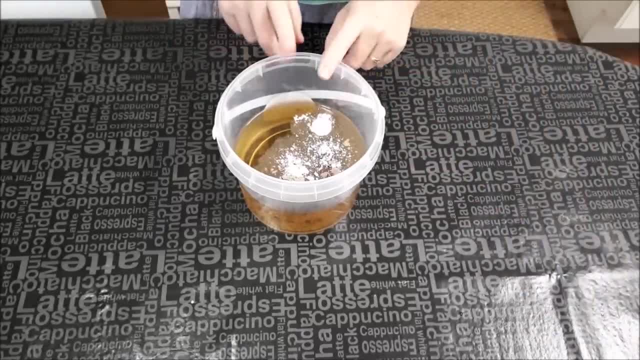 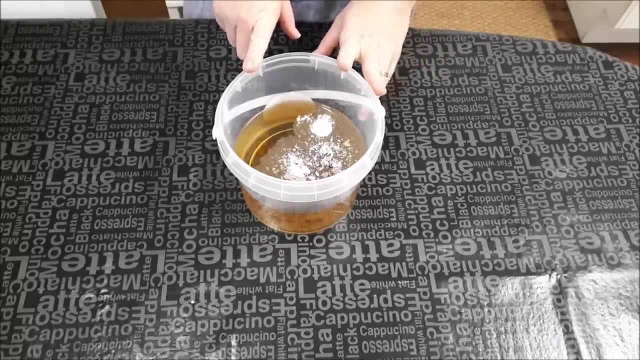 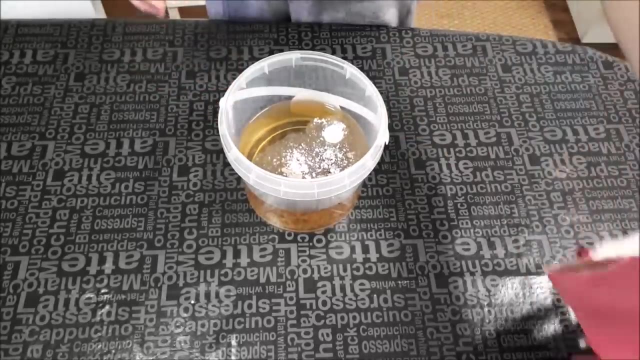 and it's more of a white color. but I like to mix all of these things in at the beginning with the stick blender, without the lye added, because then you can mix them all in to your heart's content, um, and you know, they just get really well mixed without sort of speeding up the soap at all. all right, so here we go. 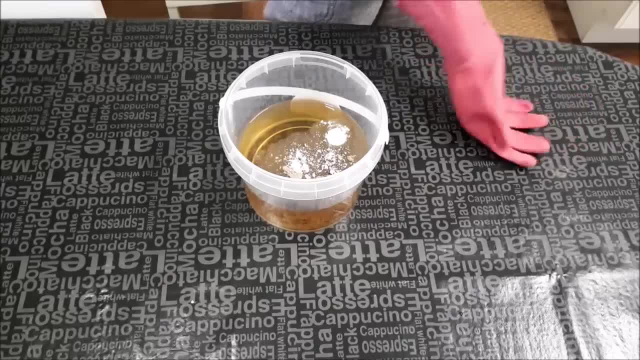 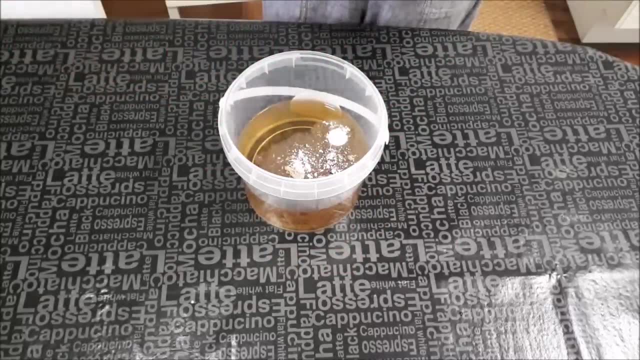 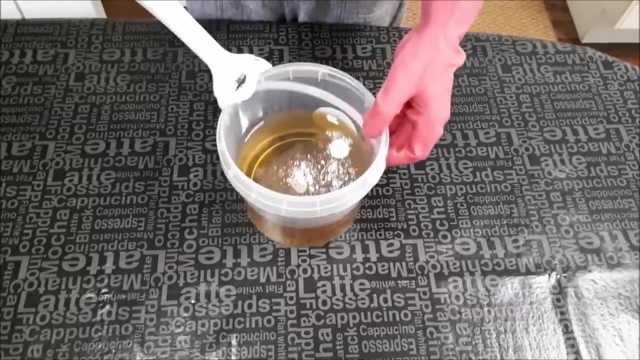 this is a bit exciting putting my gloves on, because I'm going to be handling the lye solution now, um, and I think I've got everything ready, okay. so first of all, just stick blending in these, just these little colorants. one thing is: when you're making soap, always put your stick blender and 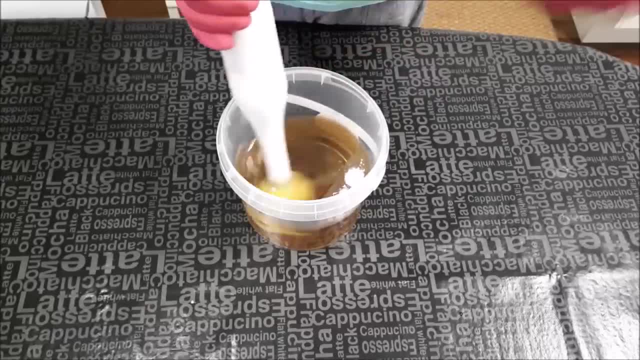 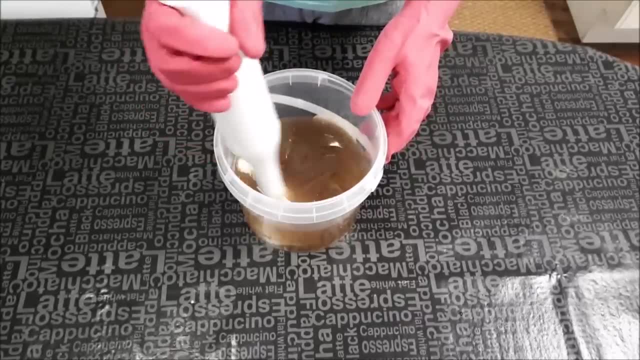 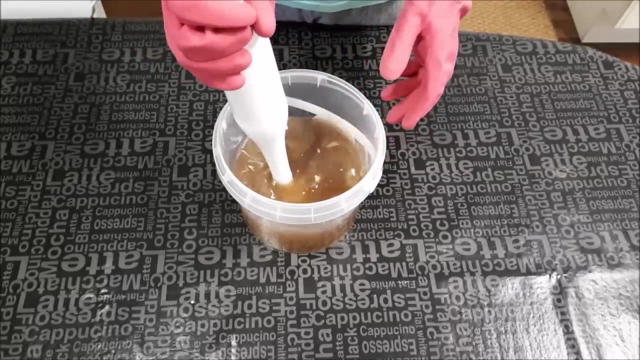 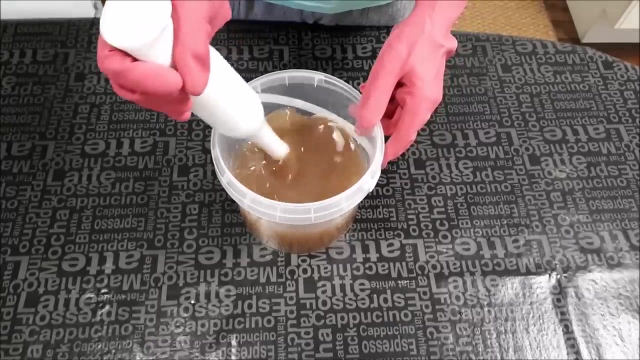 keep it under the oils. if you lift it up like that, you'll get splashes everywhere, which you definitely don't want. so just give it a bit of a stir, and sometimes clays can be hard to um dissolve in the soap. there we go, all done. 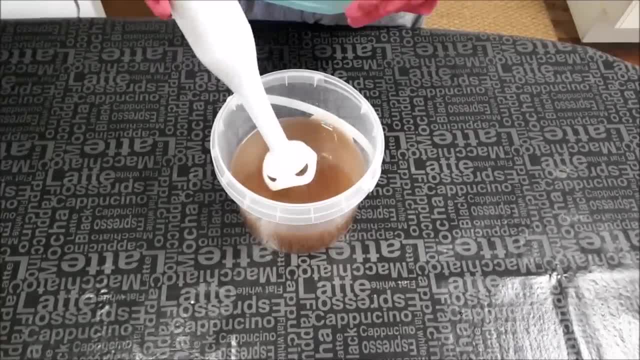 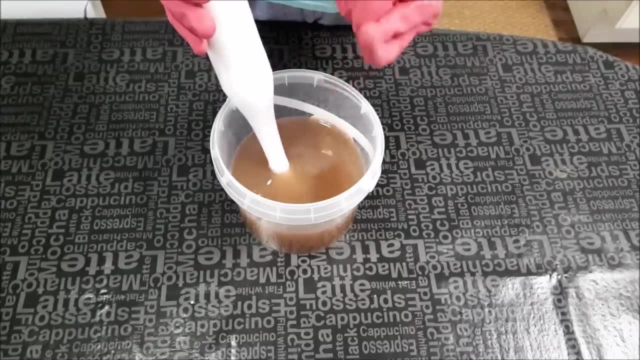 the other trick is: um, you probably saw me doing it before. when I put my stick blender in I prep, I pushed it down a couple of times. hear that sound? it basically kind of burps it, so it gets out any air bubbles that are under the end of the stick blend. 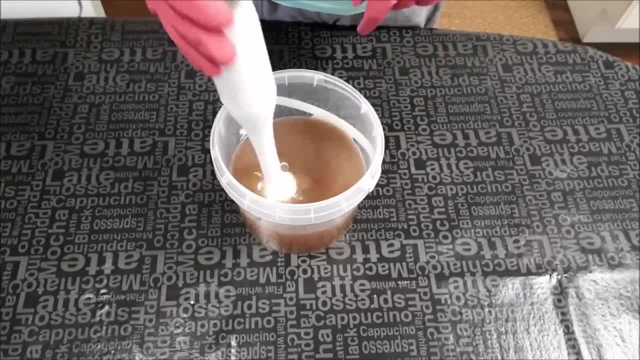 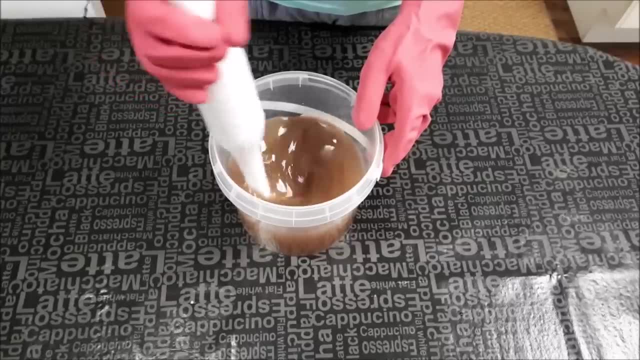 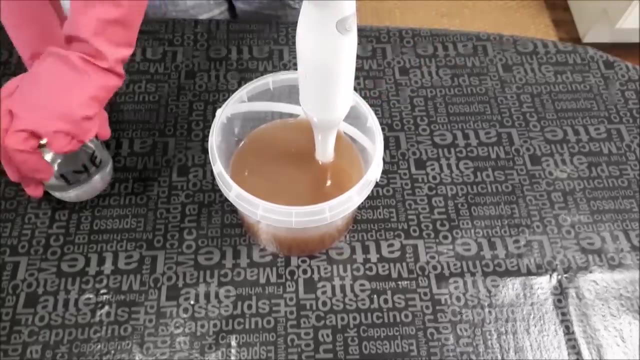 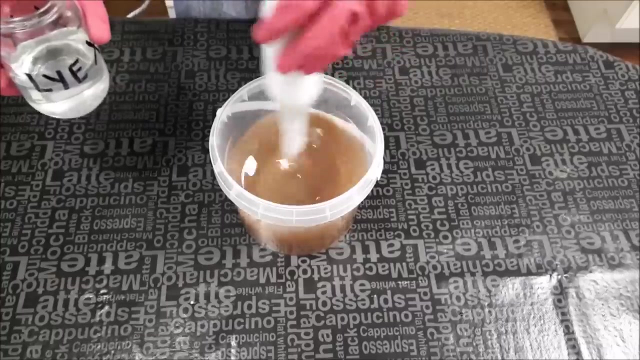 blender and that helps prevent air bubbles in your soap. so if you can burp your stick blender, that will work really well too. all right, so that's all really well blended. now I'm going to add my lye solution and just pour it. whoops, probably a good idea not to leave the stick blender standing. 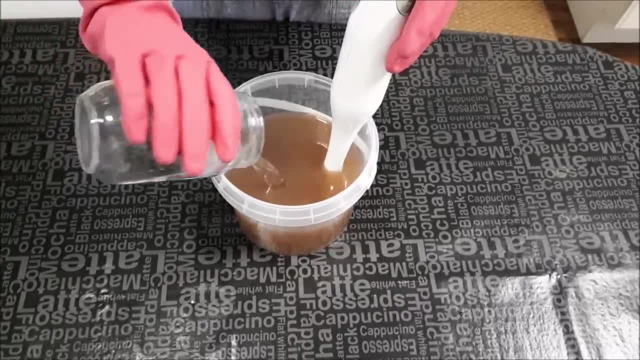 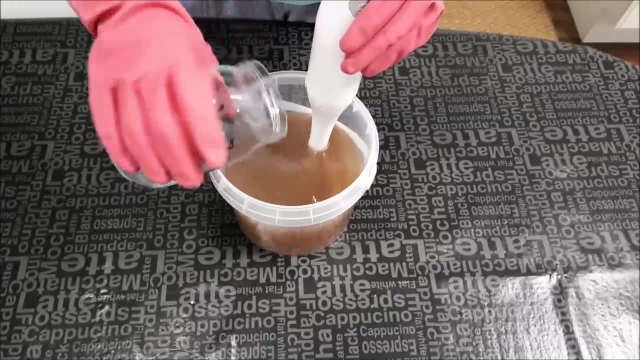 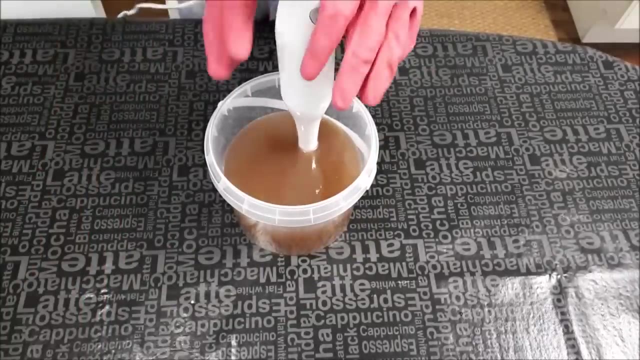 up in the bucket. so I'm just going to pour that straight in, just give it a little stir. it's not going to do anything in a mad hurry, um, but I like to get that lid back on there and get that sort of in a safe place before I do anything. 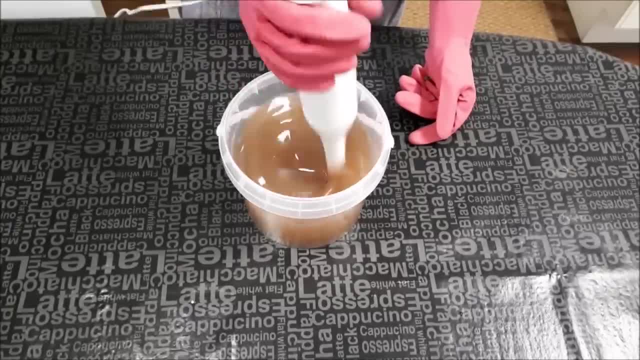 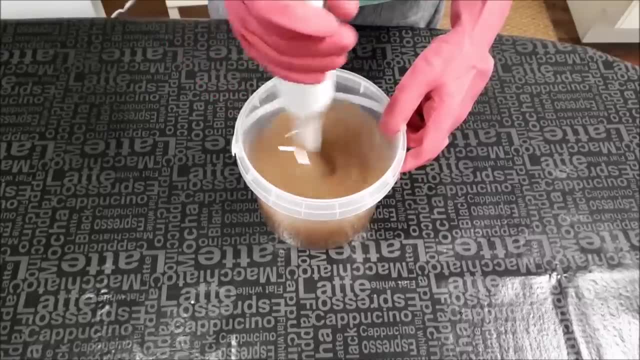 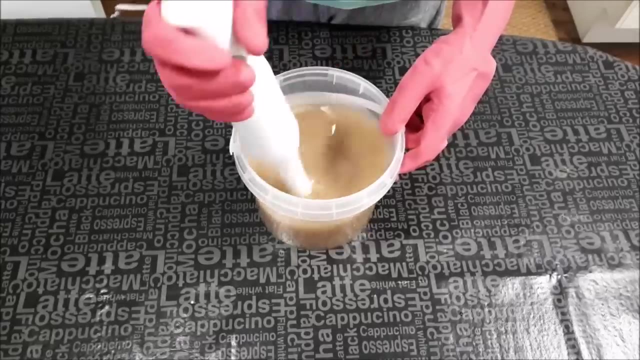 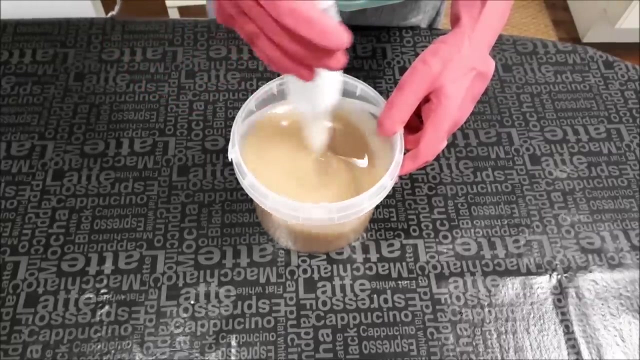 else okay. so the sodium hydroxide lye solution is in there with the oils. just start with a little mix and start stick blending to emulsify them properly. see that color change. that's what you're looking for. so olive oil soap, especially when everything's at a nice cool temperature, is fairly notoriously slow. 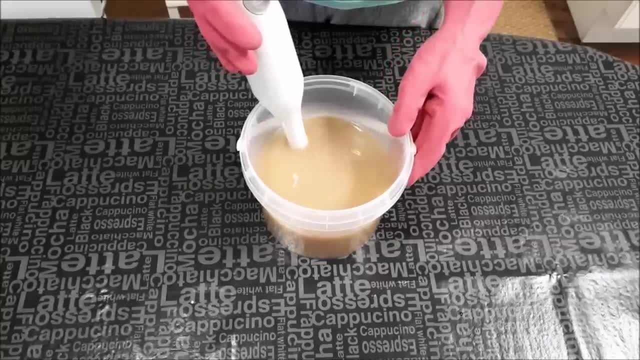 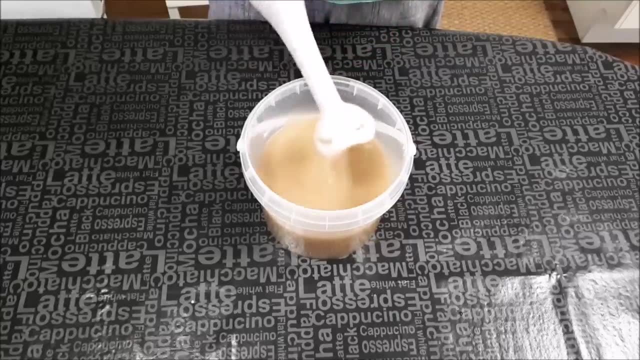 to trace. now you're asking me, I think, what is trace? trace is what we're looking for. Trace is, um, when you lift up your stick blender like that and you drizzle the soap butter over the top, I don't think you're going to be able to see it. 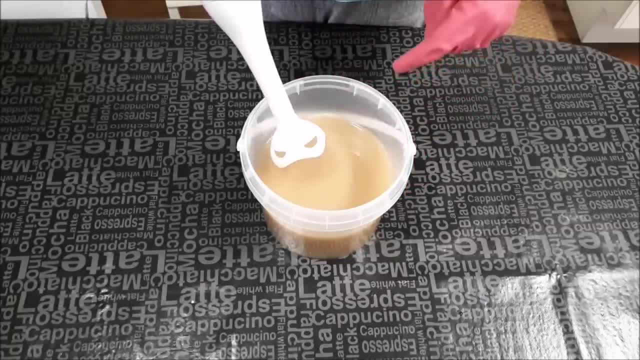 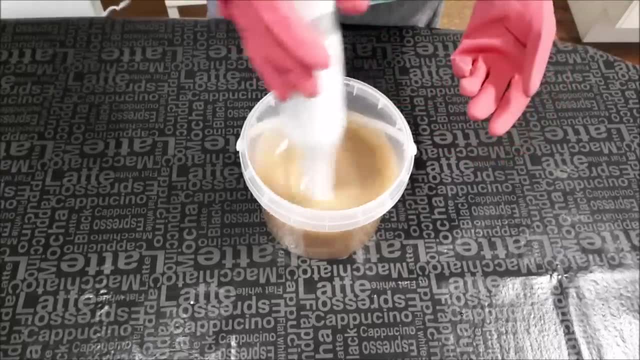 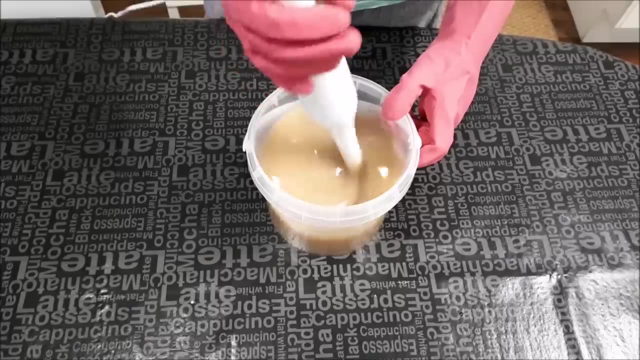 but when the when the batter leaves a trace on the surface. that's how you know when your soap batter is emulsified to a satisfactory amount. so I'm going to keep mixing and stick blending until I achieve a trace, or a light trace, if your batter has started to get thick and really gloppy. 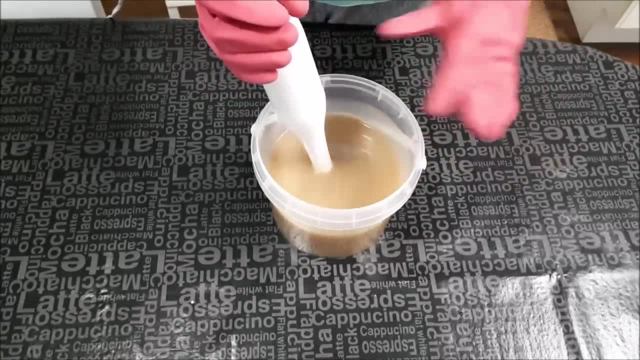 you've probably gone too far. you want just a light tray so that the batter is still nice and liquid and easy to pour in, prevent this or go bad quickly. also, make sure that what you add to the mixture to be nice and nice and a clear mixture before adding, to possibly getting� 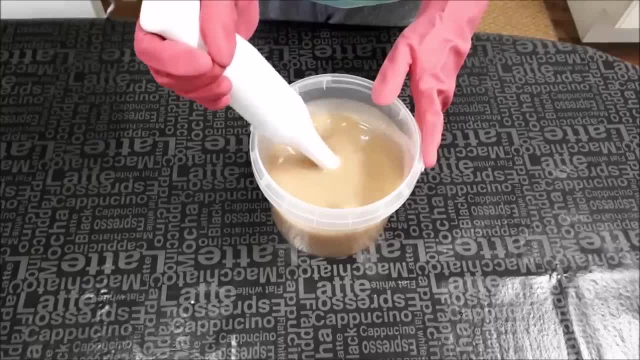 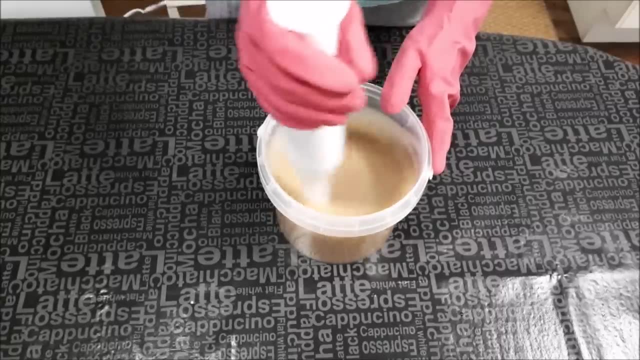 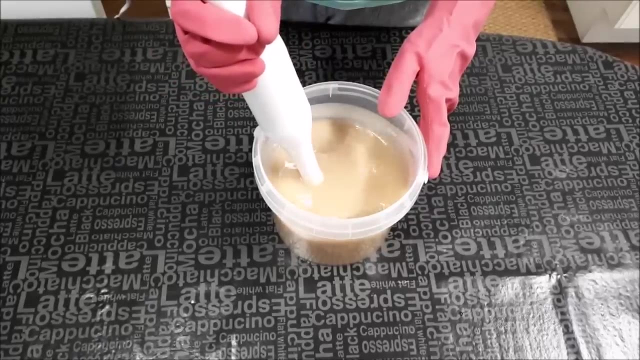 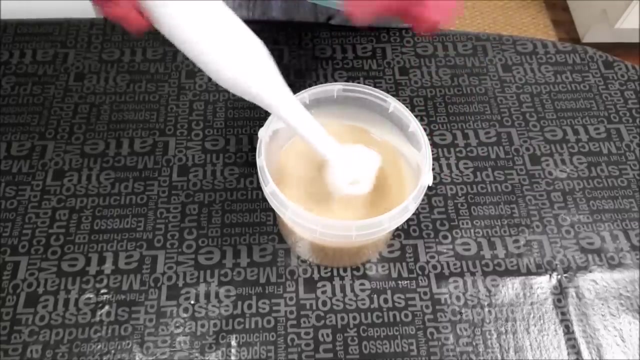 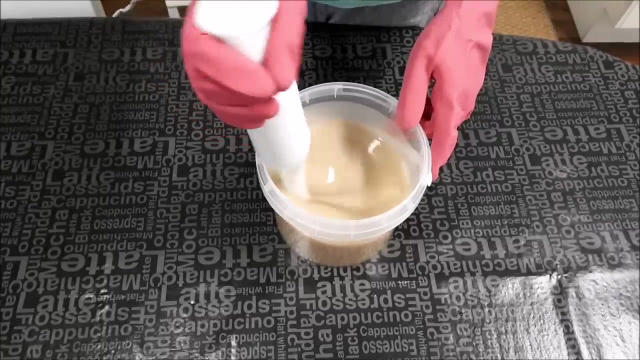 into the mold. so see how I'm keeping the blender underneath the surface all the time. I did get some air bubbles in there, but that's okay. that's getting thicker. hmm, not quite at the light trace yet. it's a nice creamy color that will hopefully be just a slight touch of. 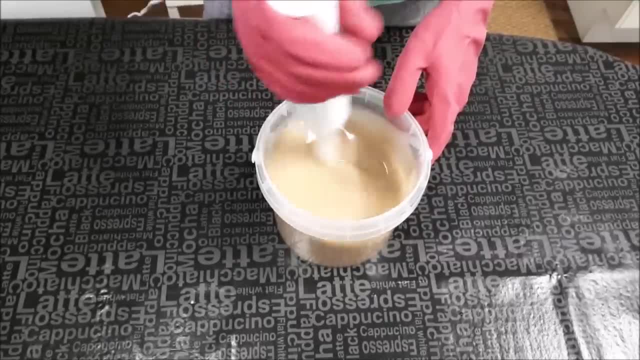 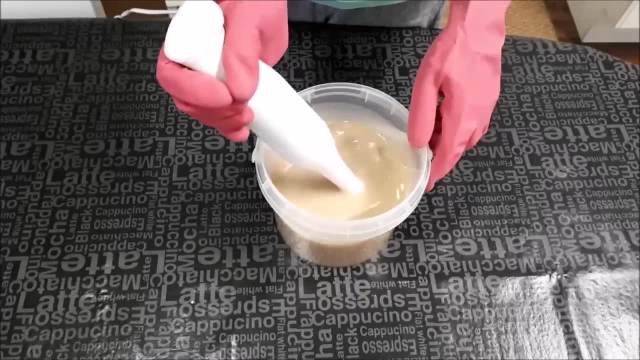 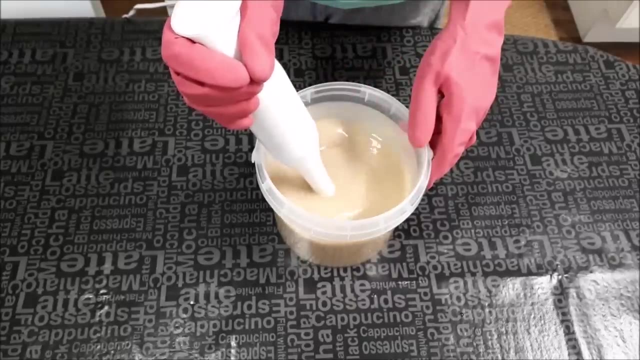 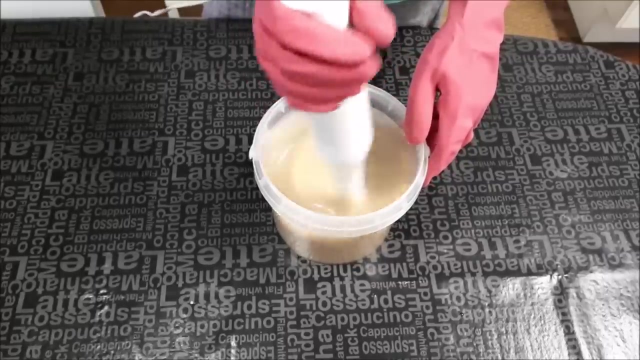 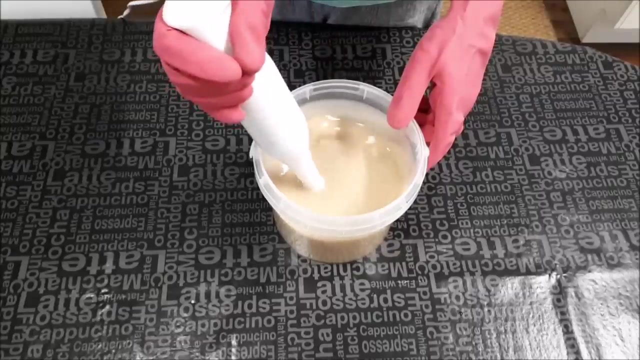 nice kind of gray pink when it's finished, not quite keep going. I often do a combination of stirring and blending, so you blend a bit and then mix that part in and then that kind of does it evenly, but not too quickly, almost if if that lye solution was really hot when I 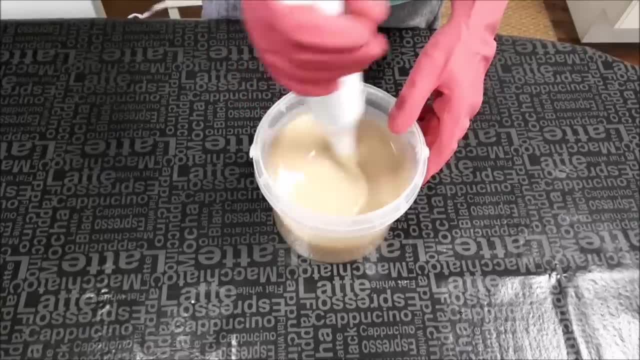 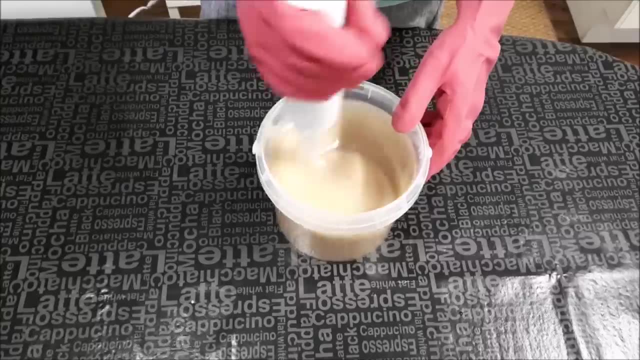 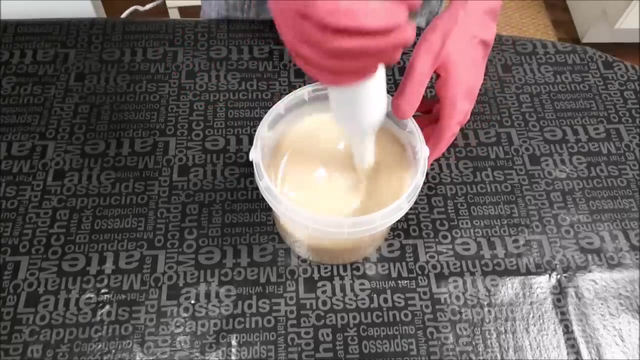 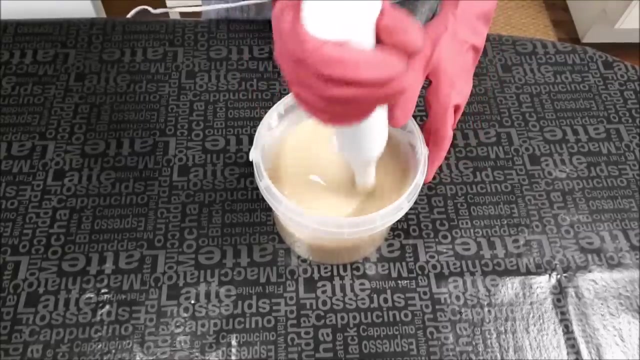 poured that in there, which is fine to do. we definitely be at trace by now. heat really does speed up the process and in fact you can make soap using another method called the hot process soap making method, where you do a similar thing but then you cook your. 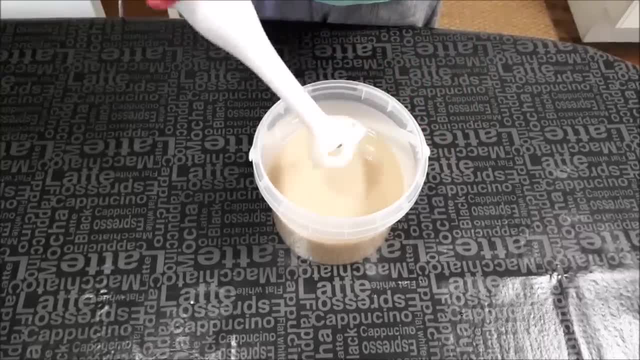 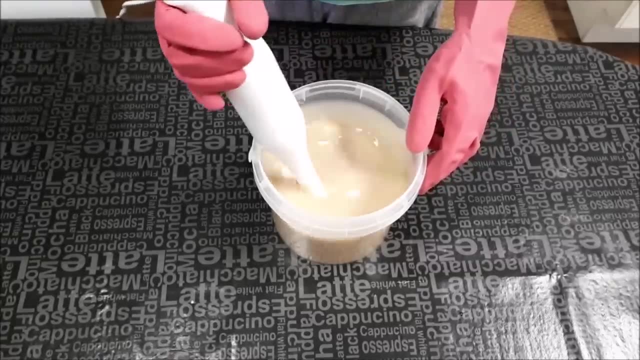 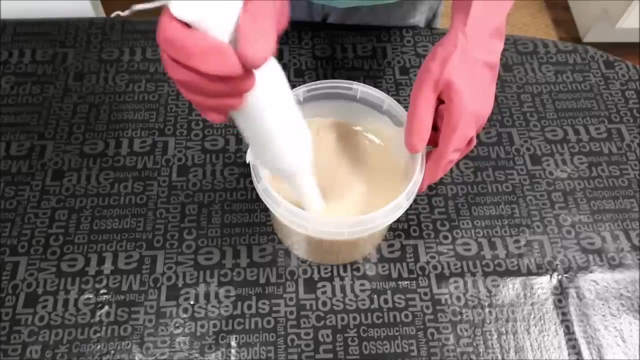 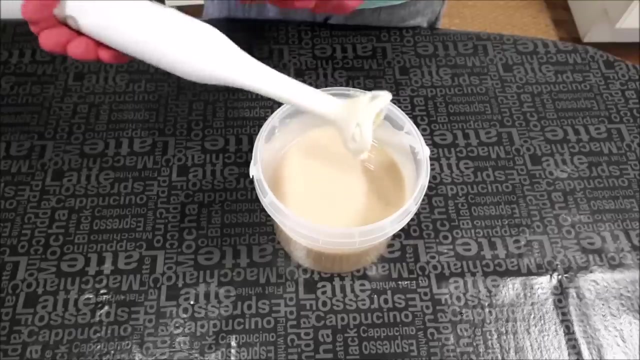 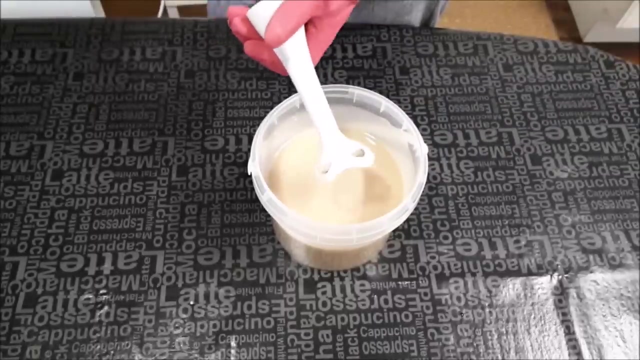 soap in a slow cooker, which is a whole different process. but you can look that up. I tend to prefer cold process method myself. I love how nice and slow this is. it's the cold method. okay, I can just see a light trace there. I'll try and show you what that looks like. I'm not going to do. 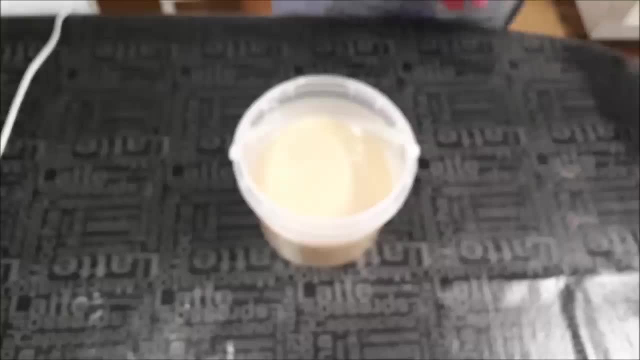 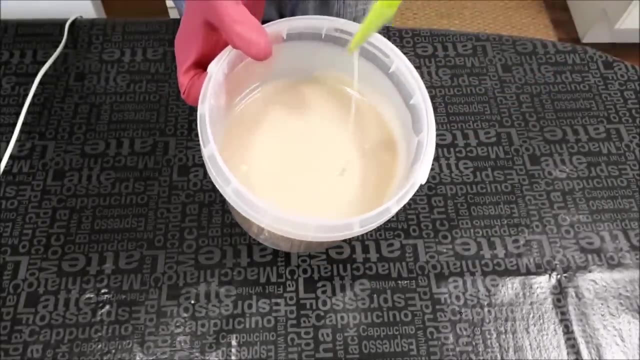 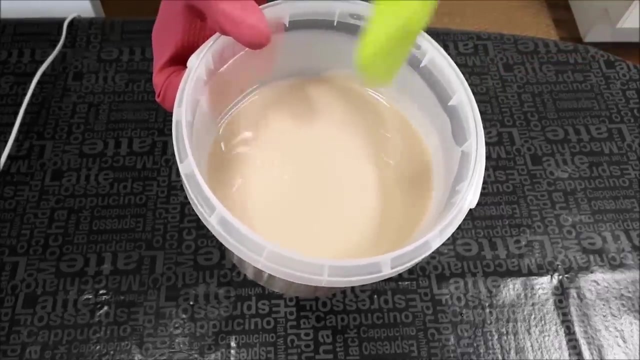 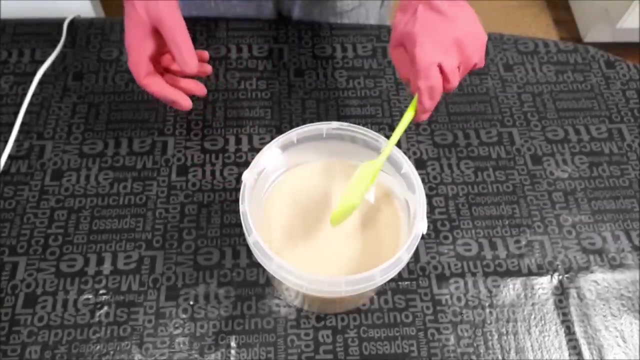 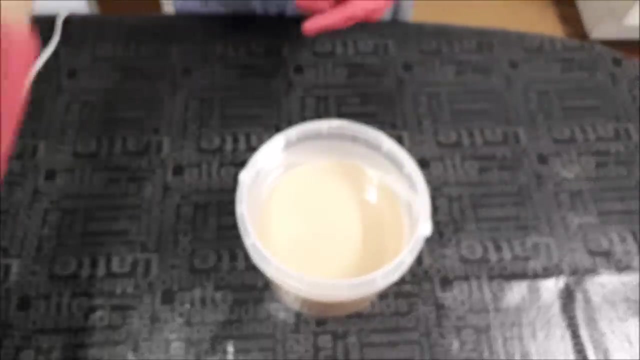 any more stick blending now. that's. that's enough. so I'm gonna get a spoon now. I don't know if you can see this, but can you see a trace of the soap butter on the surface? I hope you can. so that's a lice, a very light trace, which is perfect, all right. the next step is to mix in. 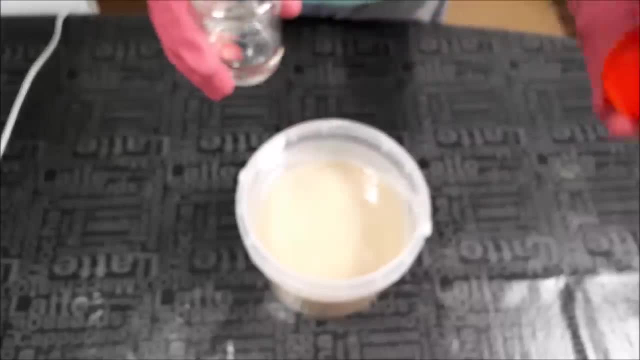 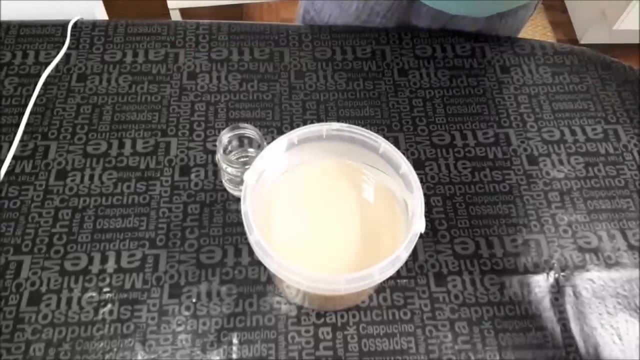 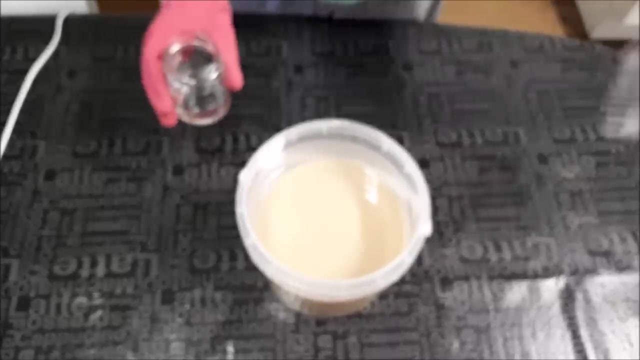 your essential oils similar to the colors. you can add this at the beginning or at the end. I like to mix it at the end because some essential oils- not lavender, thankfully, but some do- speed up the tracing process. so if they mix in at the beginning it can all go a bit quickly, so I like to just put them in at 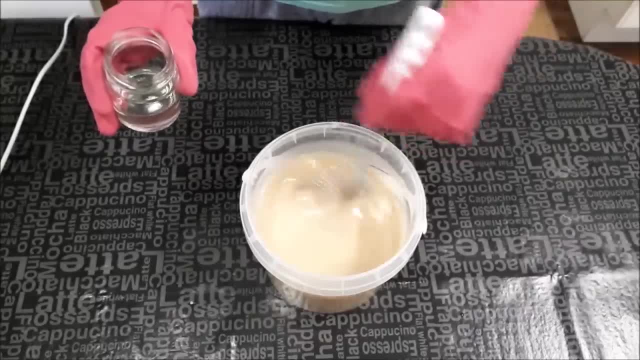 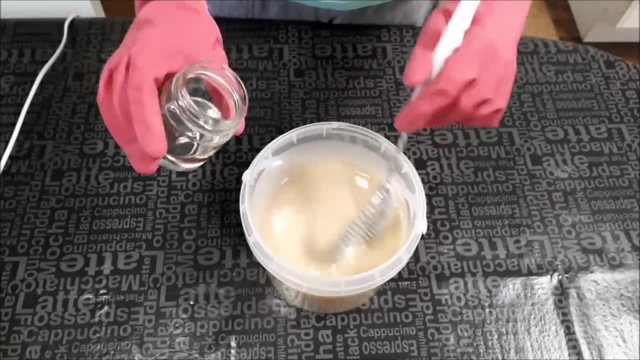 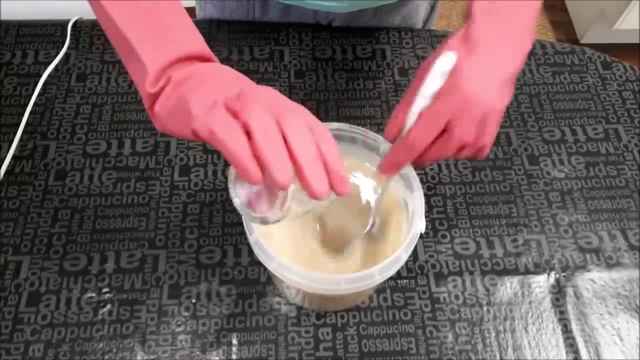 the end after I've achieved a good emulsification and a light trace. so I'm just using a whisk now I won't use the stick blender anymore- whisk to whisk in my lavender oil. so I'm just pouring that straight in and mix it through. really, really. 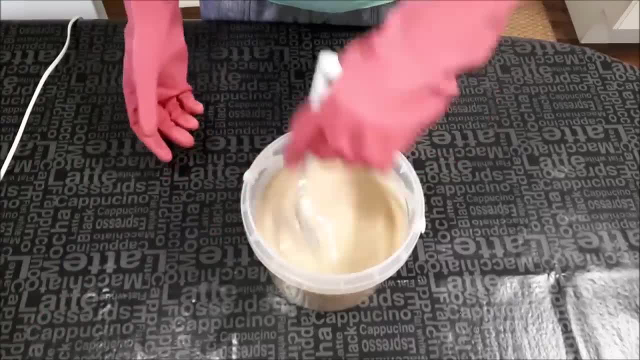 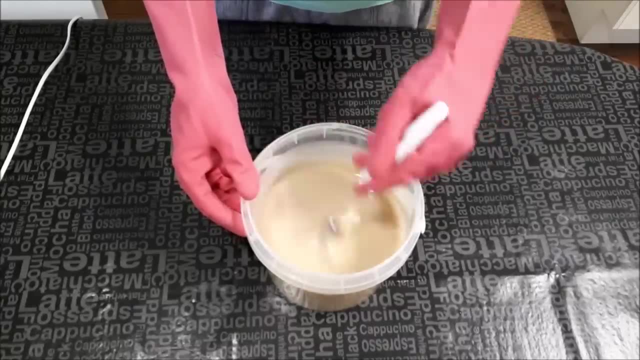 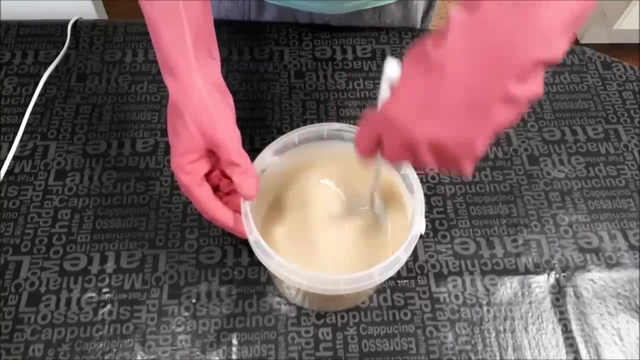 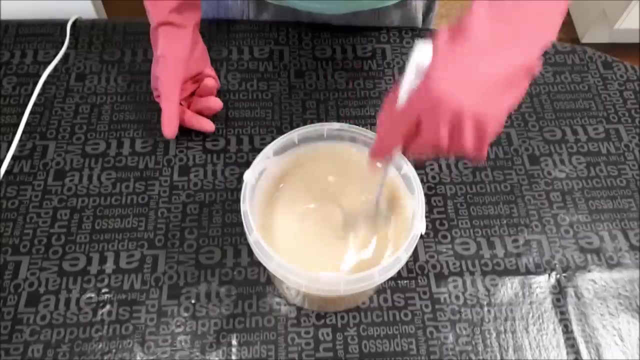 thoroughly. oh, it smells so good, lovely. now this is fully emulsified, now the soap, so it's pretty much ready to pour into the mold. the longer it sits, the thicker it will get. if you find that your batter is a bit thick and you know it's getting a bit sort of solid in the, in the 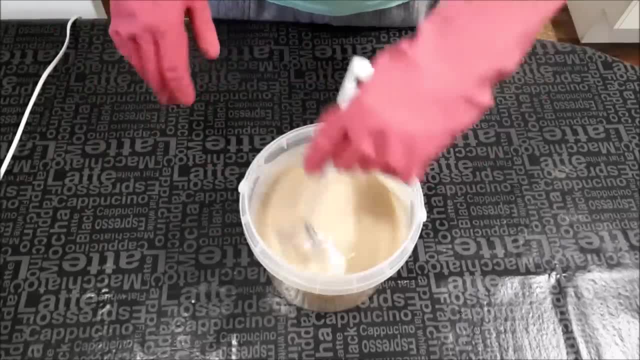 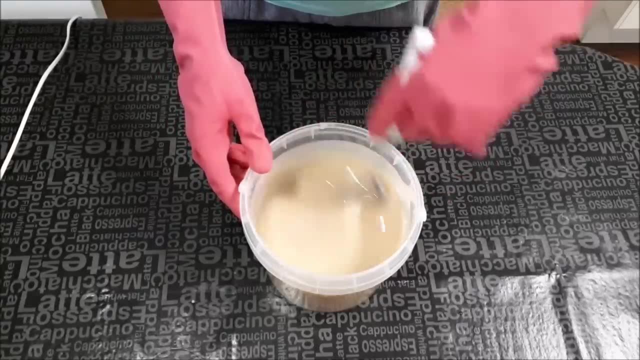 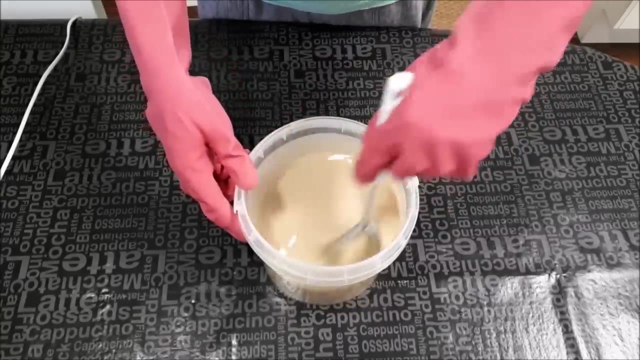 container. just give it a stir, keep stirring it, keeping it not obviously not the stick blender, because that will make it thicken up even more. but if you keep the batter moving it will sort of help to keep it a bit liquid. all right, that is ready enough for me. 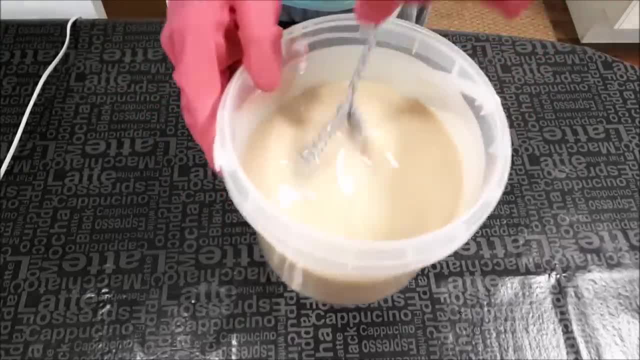 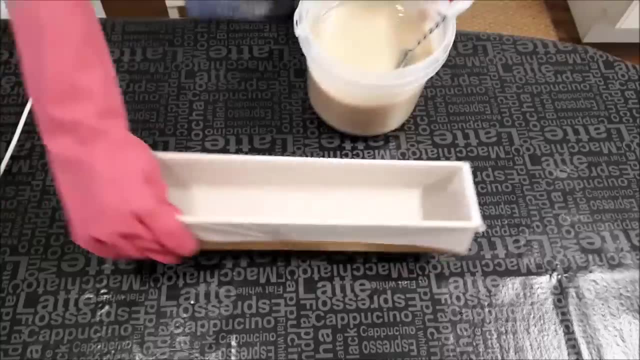 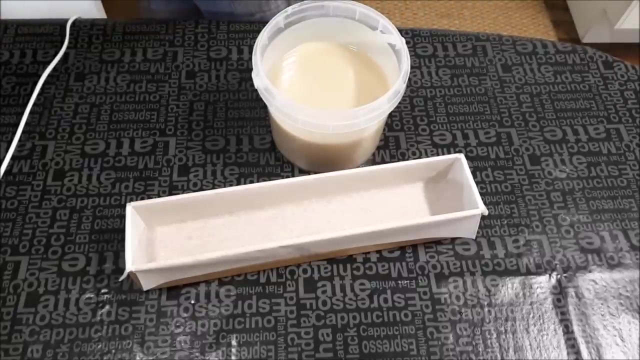 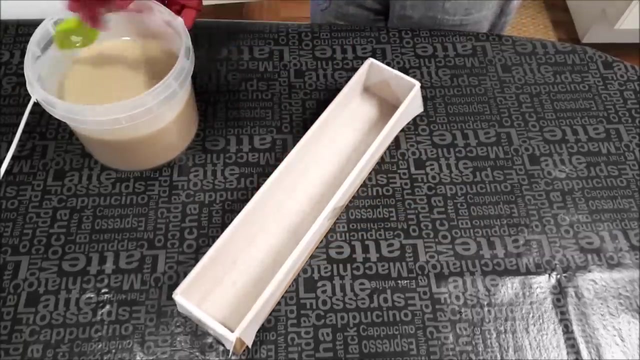 can see that. see that tracing on there. I don't know if you can see that. anyway, there's a trace. all right, now I get my mold. get rid of that one. come back to my trusty, trusty silicon spatula. these spatulas are so great. 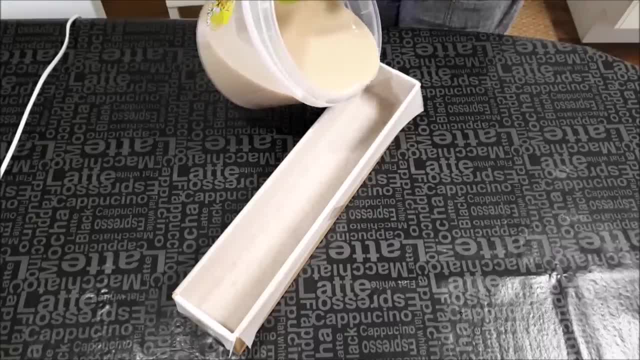 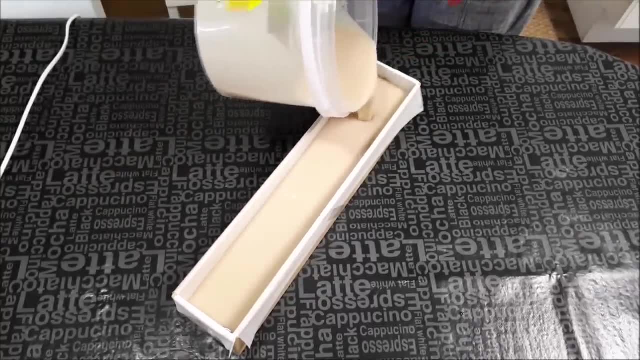 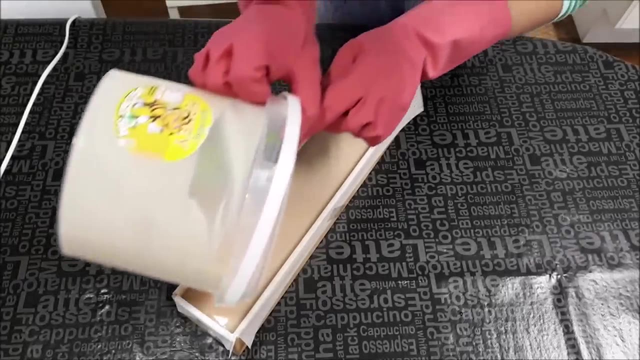 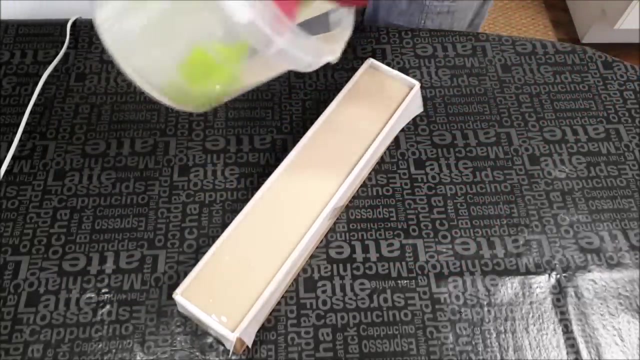 I'm just going to pour that straight in. this amount of soap just about completely fills this mold, so it's going to be very, very full, but it does fit just okay. because that's so full, I'm just going to spoon the rest in, scrape down less size. 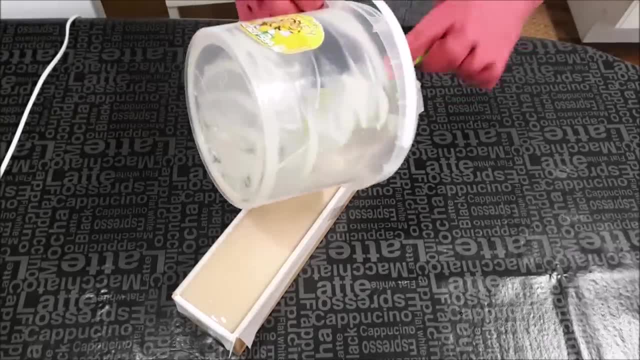 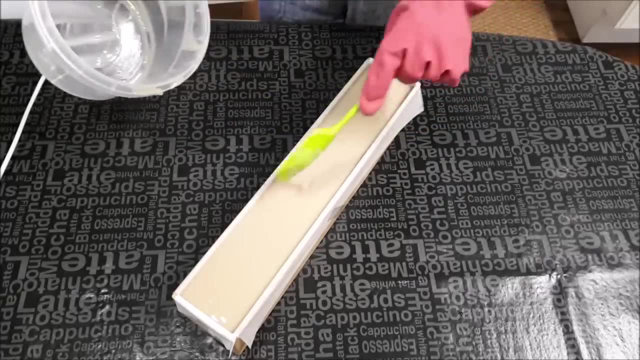 I'm just going to pour that straight in. I'm just going to pour that straight in there. now, if you want to do a fancy top on your soap or do some swirling and things, you can leave it for a few minutes and it will. it will get a bit. 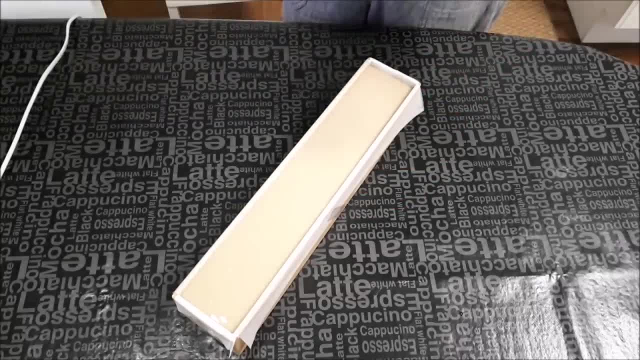 thicker, and then you'll get a bit of a pattern. I'll show you what I'm going to do. sometimes I put lavender buds on the top of this lavender soap, but I'm not going to do that today, Jordy. Awww, maybe it will. 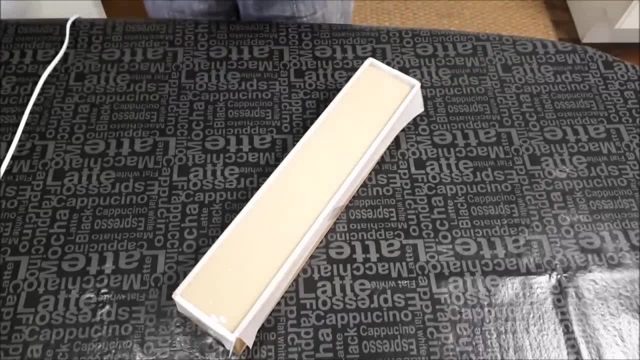 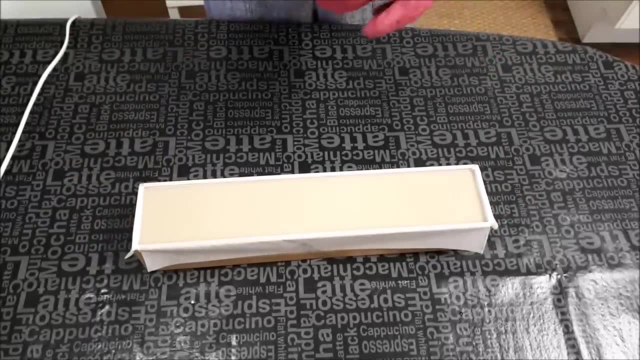 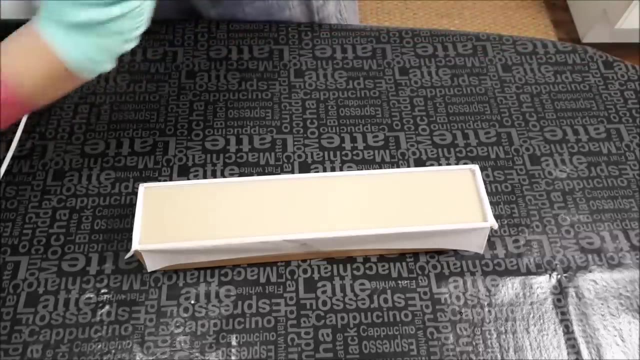 No, I'm just going to do a basic swirly top with a chopstick. so there you go. you have one batch of beautiful cold processed olive and coconut oil, soap with lavender essential oil and, to finish it off, I'm just going to get my 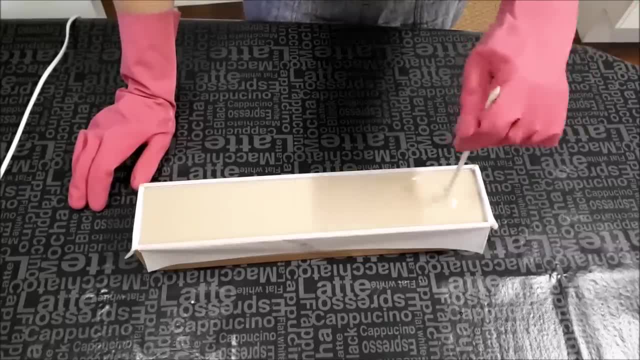 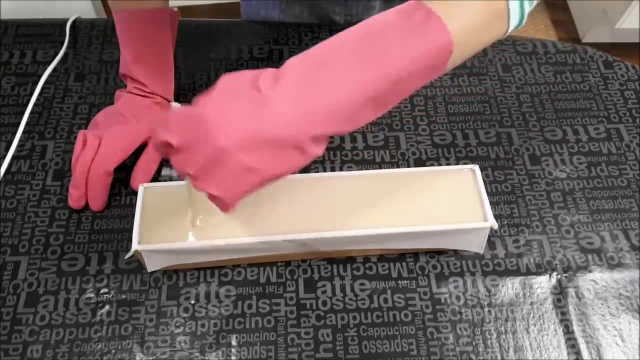 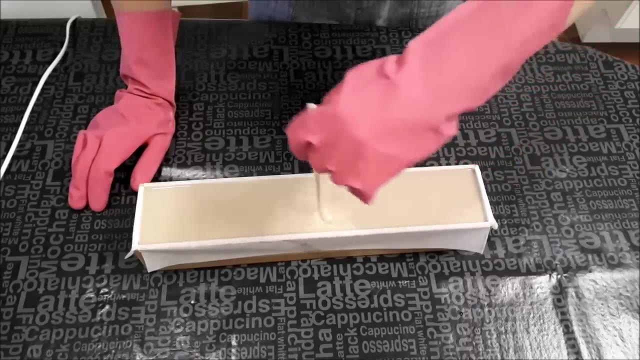 chopstick and just do some light little swirly patterns. you probably can't see them too well. what this does to to is if you've got any lumpy bits on the top, just giving it a swirl with the chopstick just sort of helps smooth it. 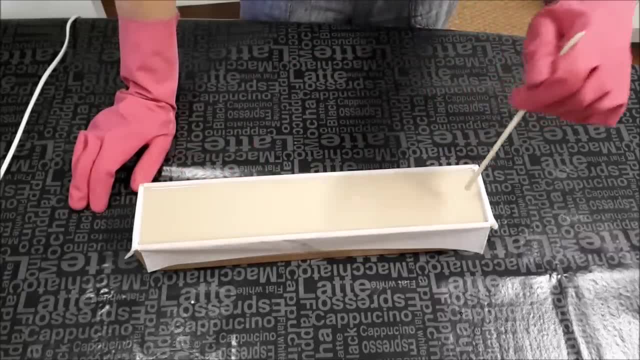 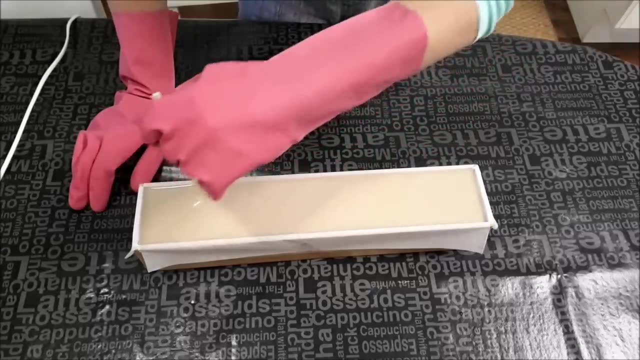 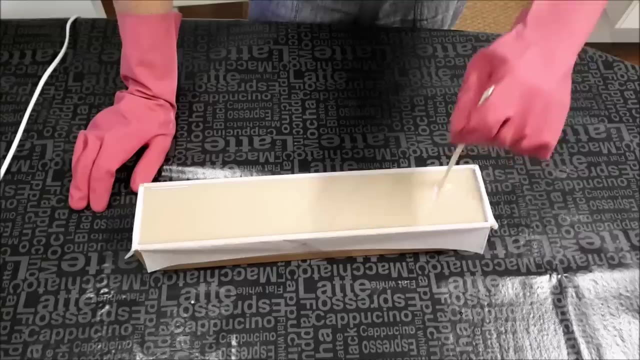 out. but this is quite liquid so I'm not really getting any pattern in there. you can do this kind of pattern to do all sorts of patterns. obviously this soap is still very liquid. once it thickens up a bit you get a bit more pattern and do that sort of thing. I personally quite like the little. 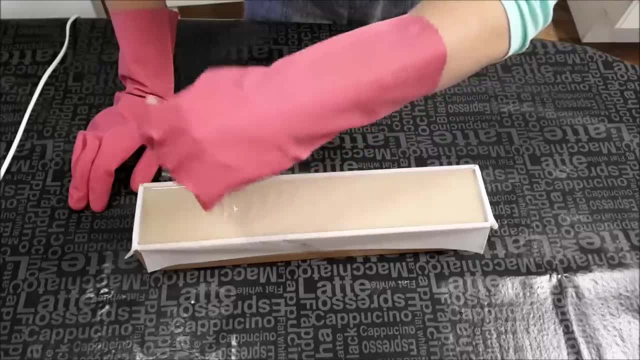 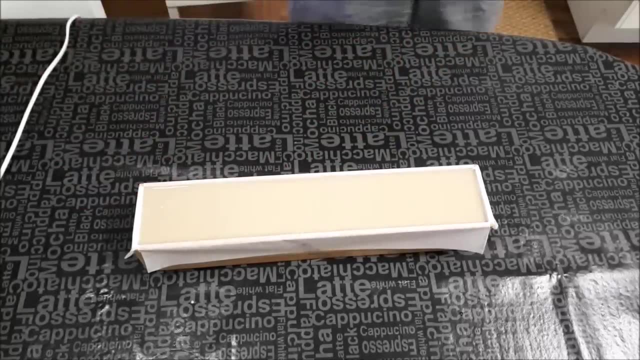 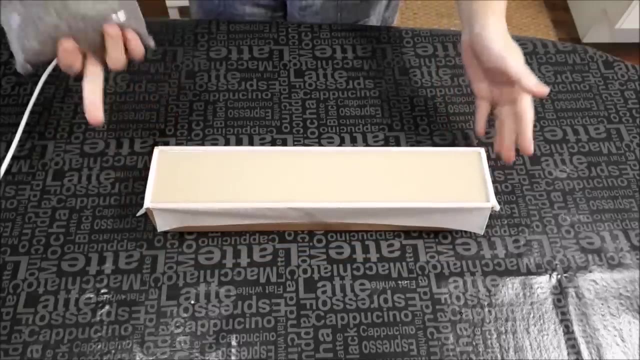 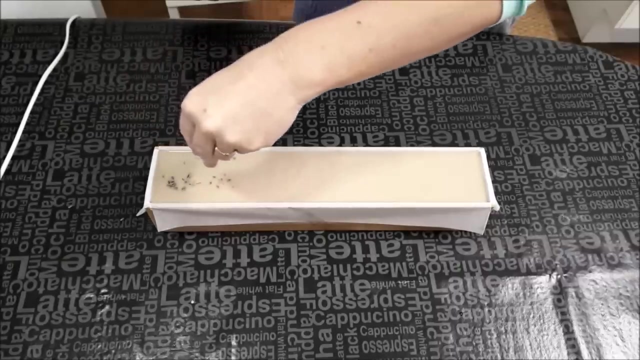 circle, these swirls like that. I'm going to leave that as it is very plain. okay, that's it. I'm back again. I decided I would put some lavender essential oil soap on top of that, and then I'm going to do a little bit of that just to get that nice and smooth and smooth. I'm just going to 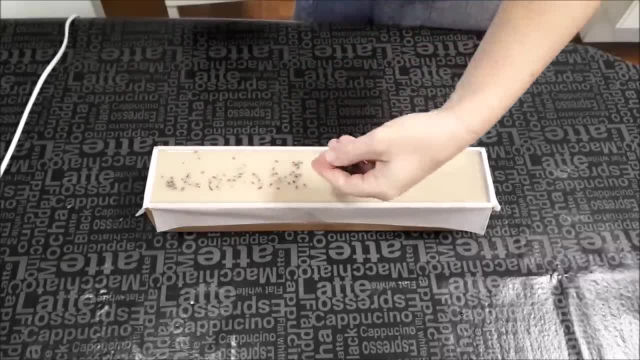 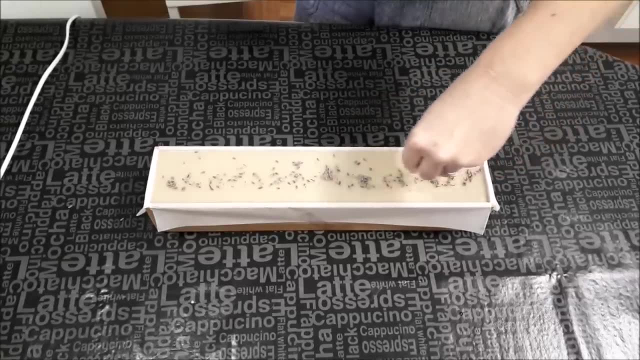 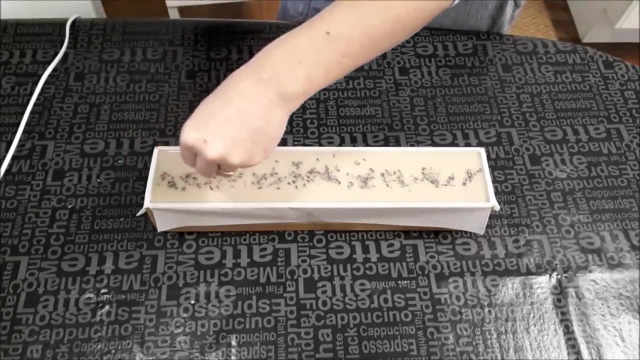 sprinkle a little bit of lavender essential oil soap right here on the top, and I'm just going to take a little bit of lavender essential oil soap and I'm just going to sprinkle a little bit of lavender essential oil soap right here on the top. you can mix these into your soap as well at the end, but any 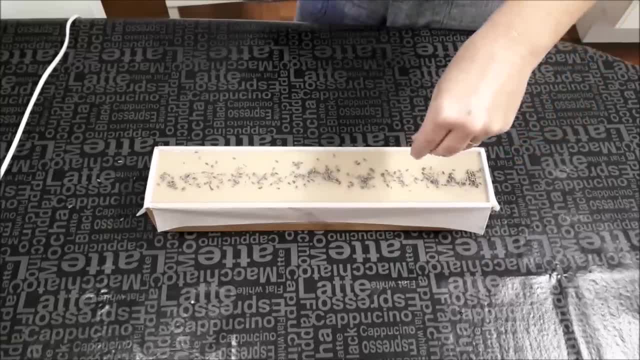 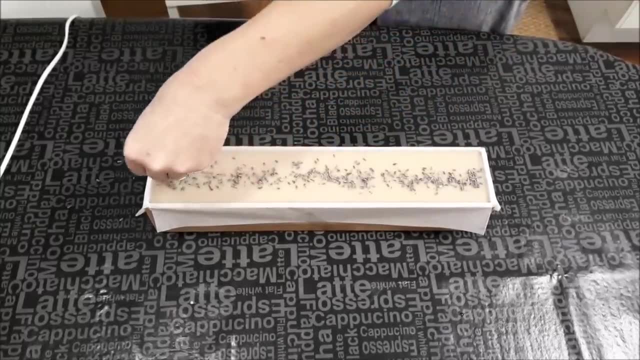 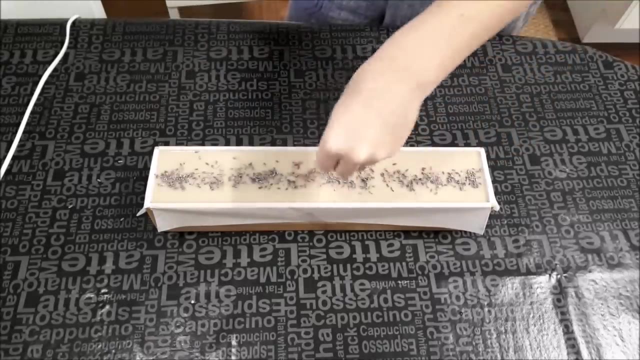 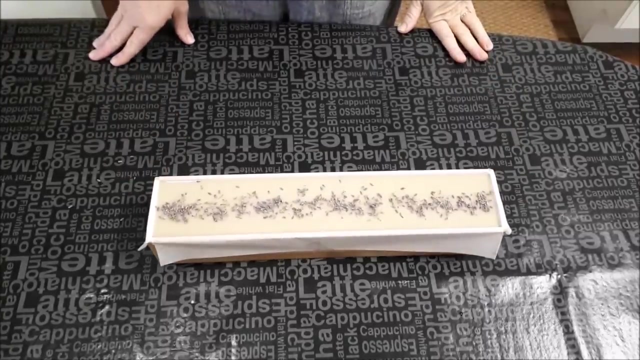 botanical ingredient tends to go brown in the soap during the saponification. so top is a better option. better option, there you go. that'll do a little bit more. sprinkle, sprinkle, sprinkle, you do whatever you like. okay, there we go, beautiful soap. I will put this away now. I should tell you that, wrapping up your 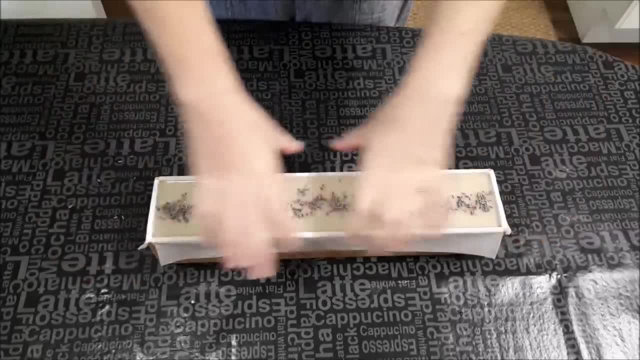 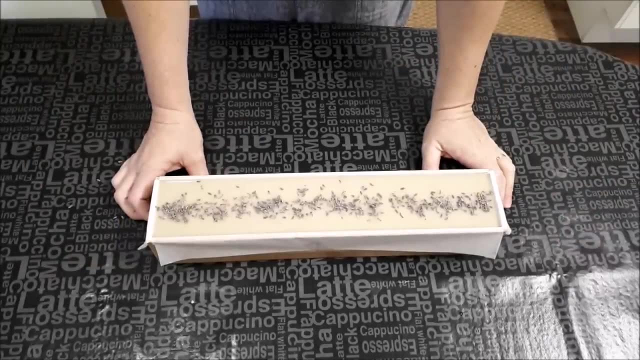 soap is really good, so I'm just going to put a piece of cardboard over the top and then I'm going to wrap it in a towel and what that does, or a little blanket, and what that does is it helps the soap to heat up. it will heat up as it. 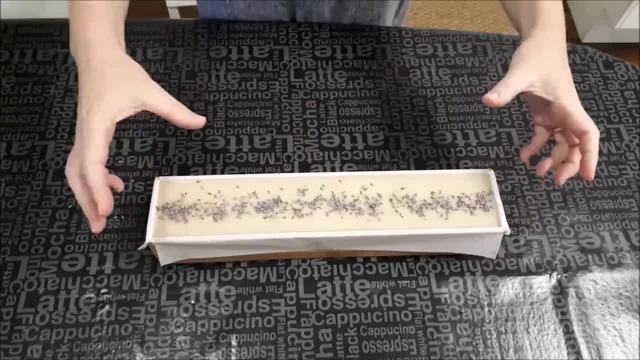 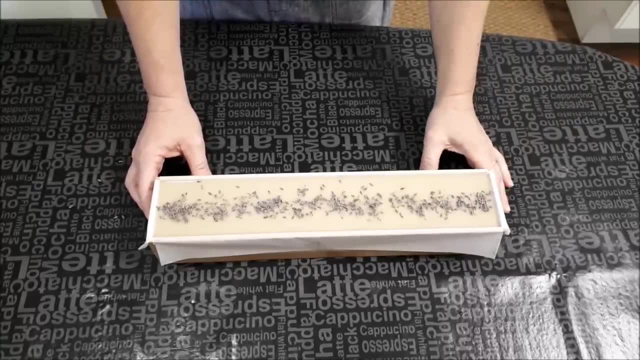 saponifies and hardens and you want it to heat up evenly. if you don't let it heat up evenly, you get sort of a central part of the soap that's a different color to the outside and that's because it goes through a gel phase. so the soap 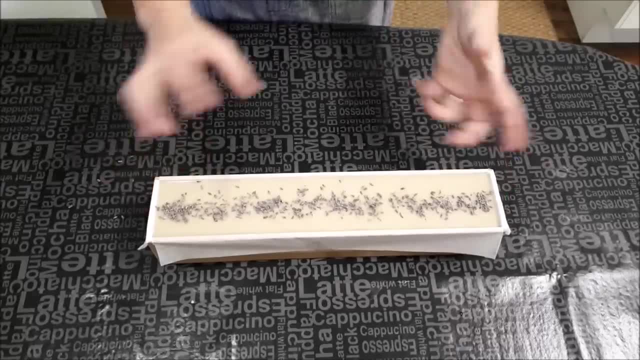 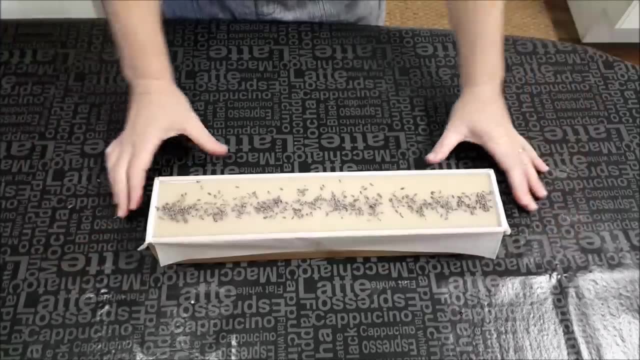 will. if you take a little bit of soap and you take a little bit of soap and you take a peek, you will see that the soap goes through this funny jelly phase before it turns solid again and you want to get a really nice full, even gelling. 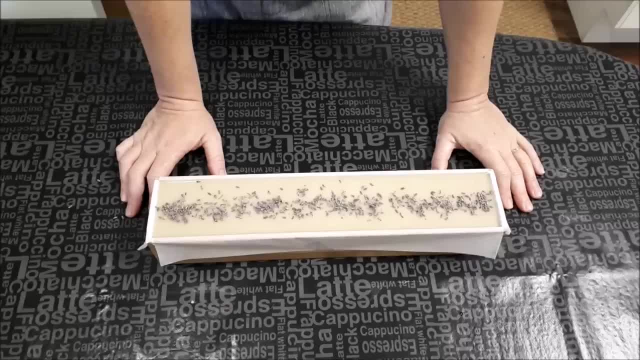 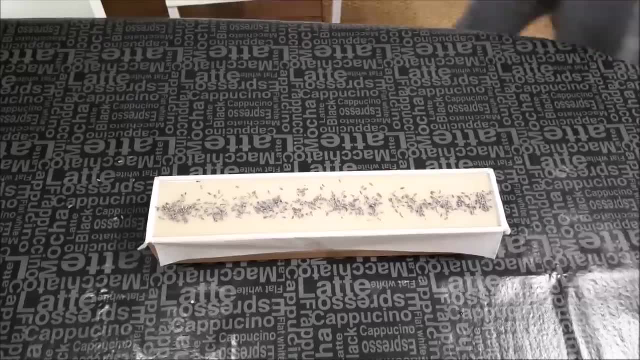 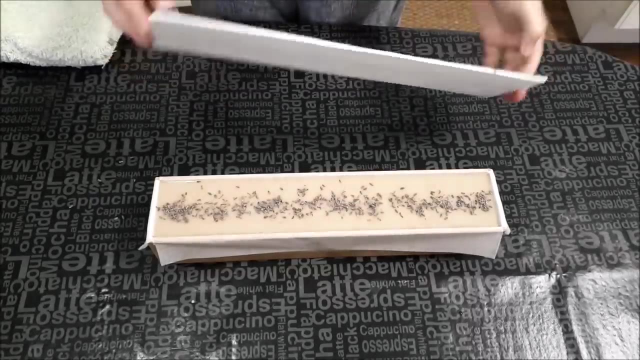 of your soap. so the way to do that is to insulate it just by wrapping it up. so I'll actually do that and I'll show you how I do that. so to wrap your soap up for insulation, I've actually got this piece of corflute which is just from an 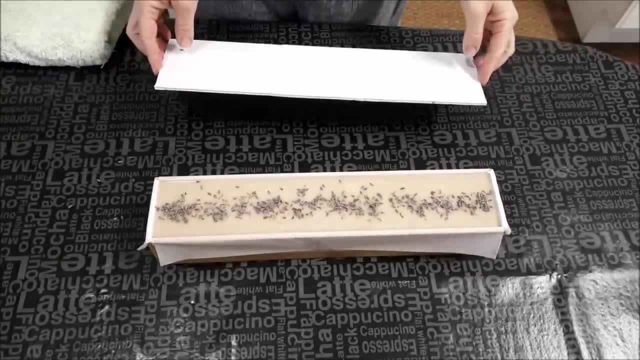 old election sign. I've actually got this piece of corflute which is just from an old election sign. that's really good. or a piece of cardboard is good, depending on how full your soap is in the mold. this one's really full, so I'm gonna have to be a. 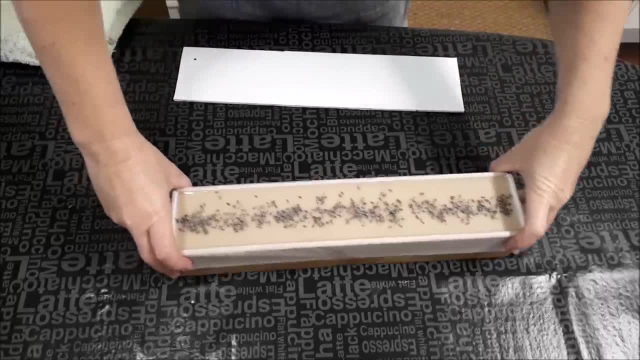 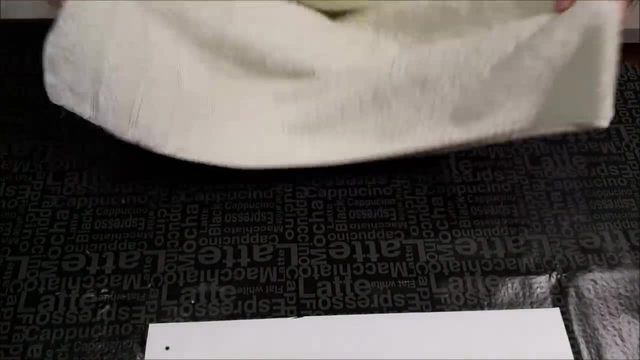 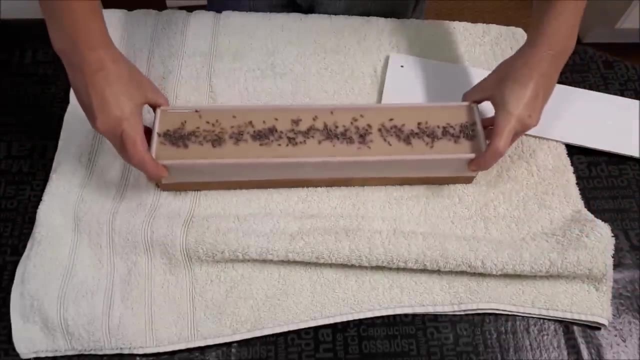 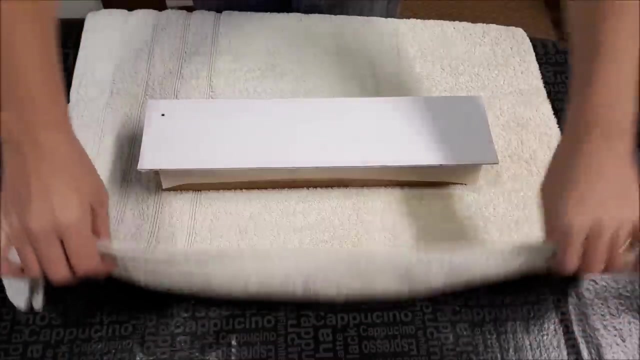 bit careful with it, but basically I'll put that aside. actually, so you just need an old towel and then put your soap- it's already starting to thicken up, I can see it's not quite so runny- and then cover it up, just so the towel doesn't go into the soap, and then you just wrap it up in. 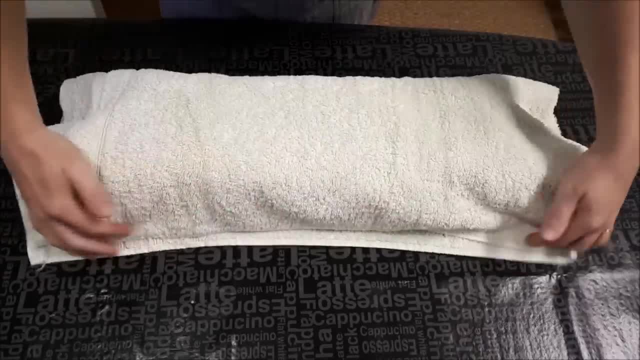 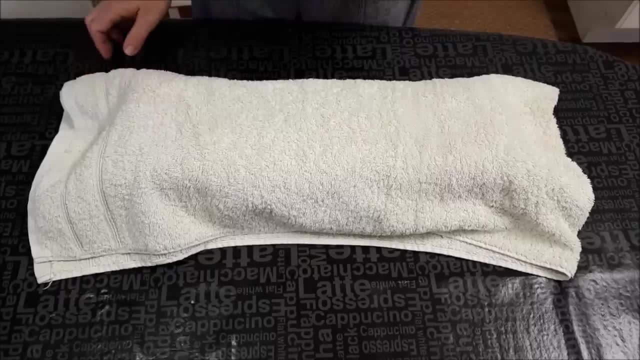 winter you can use- you know, you can use- a woolen blanket or something quite warm. in summer, just use a towel or one layer, because if it gets too hot it can overheat and expand a little bit, which you don't want, so just just wrap it. 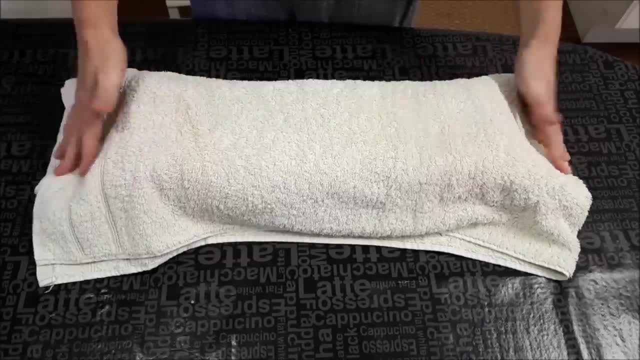 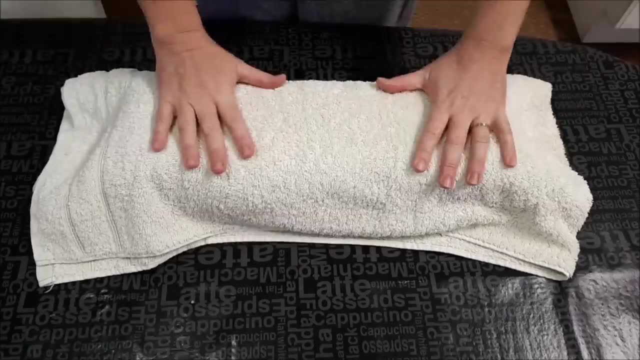 according to the season, but that's going to be enough for this soap, and it's fairly cool here. it's June in Brisbane, so oh, it's May in Brisbane. anyway, there you go, so I will come back 12 hours later and it will be ready to cut. it should look. 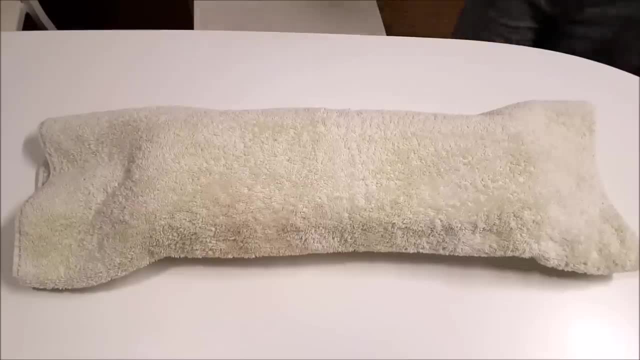 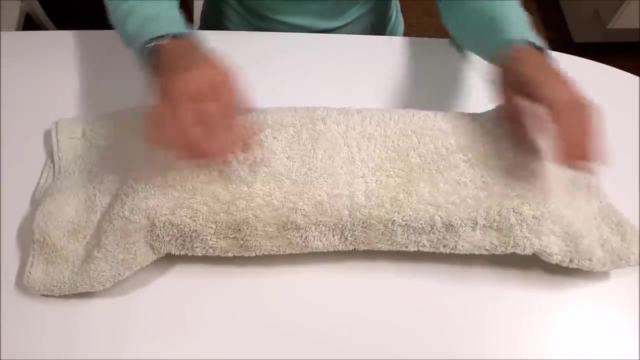 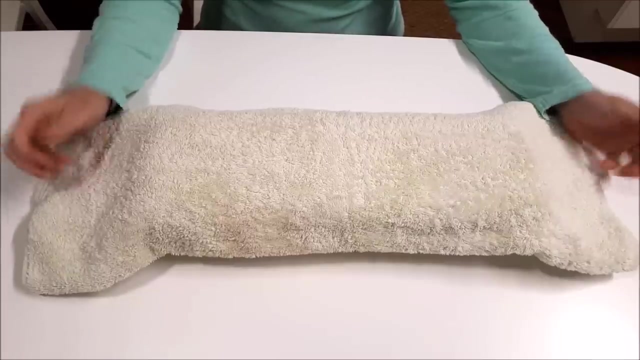 really good. well, here we are. it's about 5: 30 pm, so it's about eight and a half hours after I made this soap. in the recipe I say that you can leave it for about 12 hours before you cut it, but anywhere between 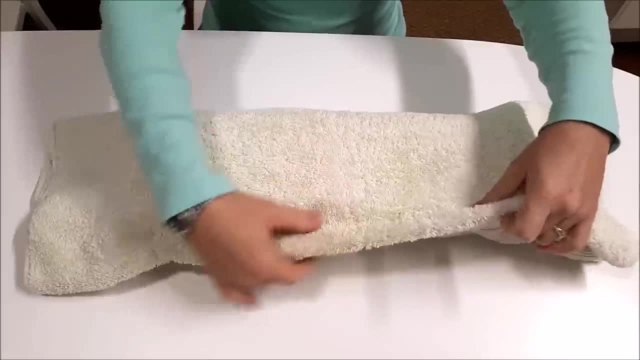 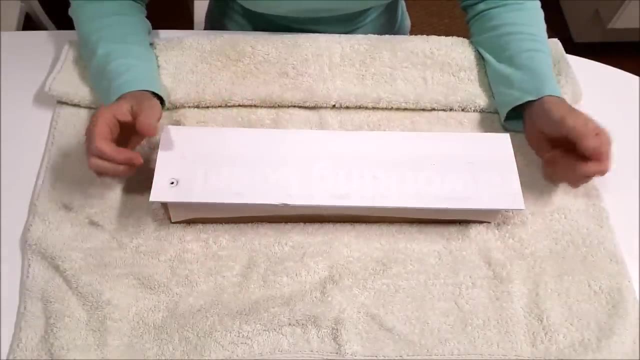 eight and about 15 hours. it's okay if you leave this soap for 24 hours. it might be a little bit too hard to cut and that's because of the strong lye concentration. it has quite a low amount of water in this recipe, so here's the 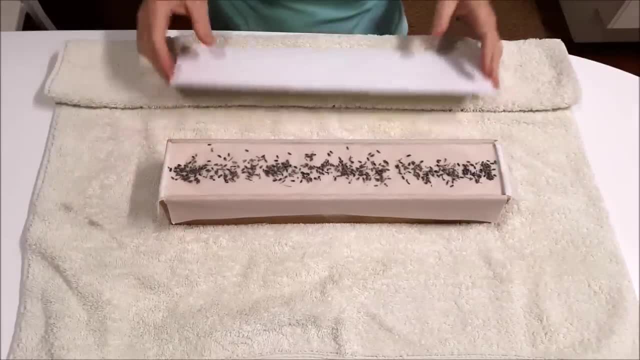 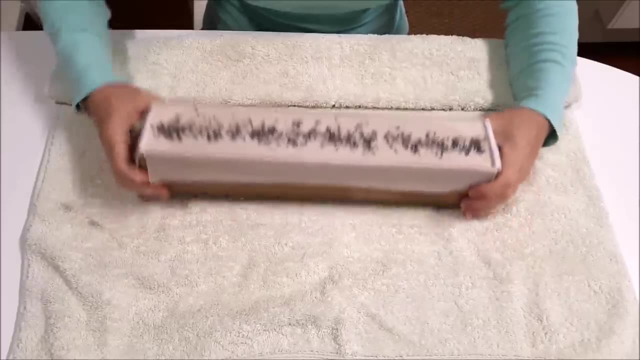 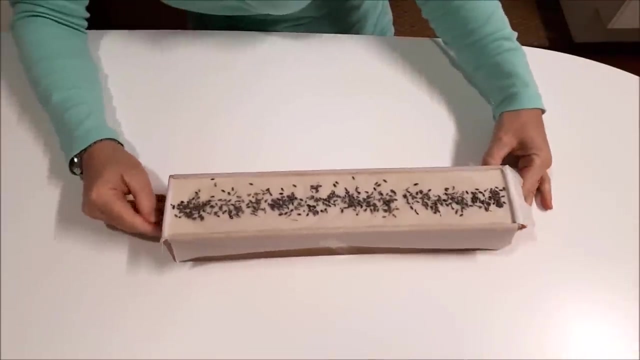 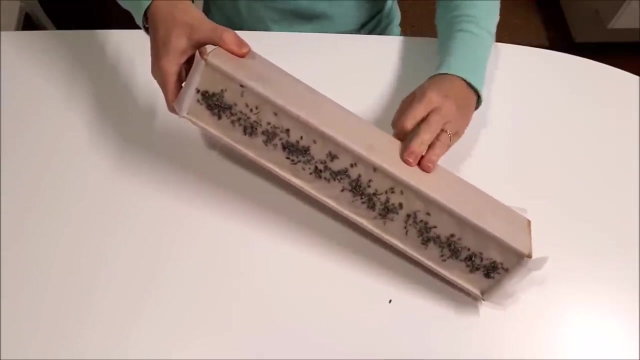 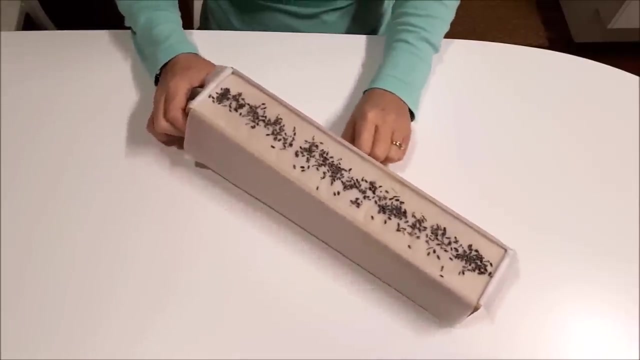 soap. it's been through its gel phase and it's ready to cut. it feels quite, feels quite solid actually. so I'm just going to take that towel out of the way and take off the sticky tape. looks like I actually got a partial gelling of this. 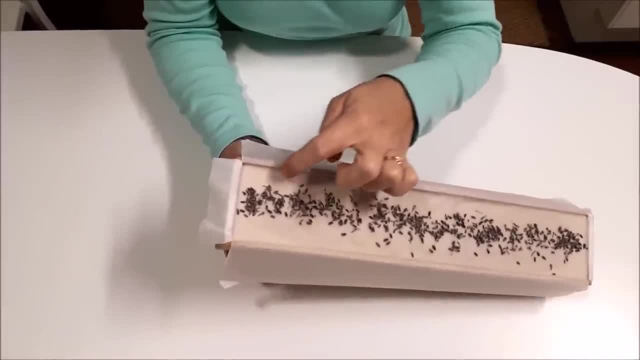 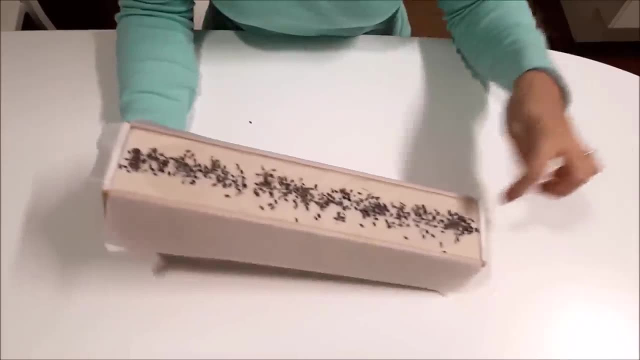 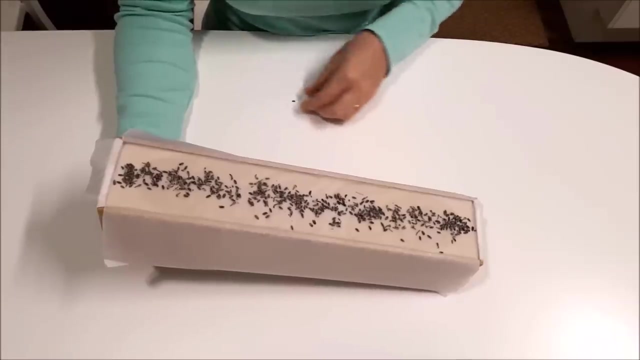 soap. I don't know if you can see that that line shape. there, where the end of the soap is a lighter color than than this part, there is a bit of a round shape which suggests to me that it didn't gel all the way to the ends. so I may have needed to wrap the soap up a bit more. but 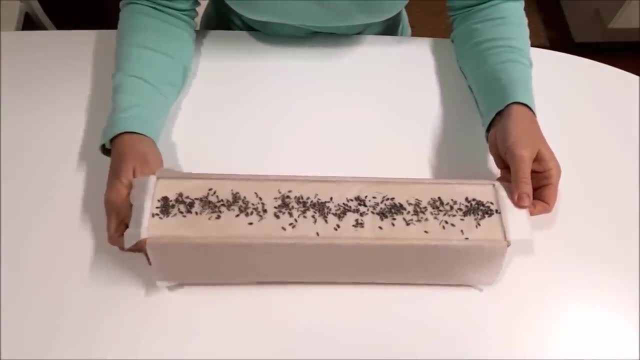 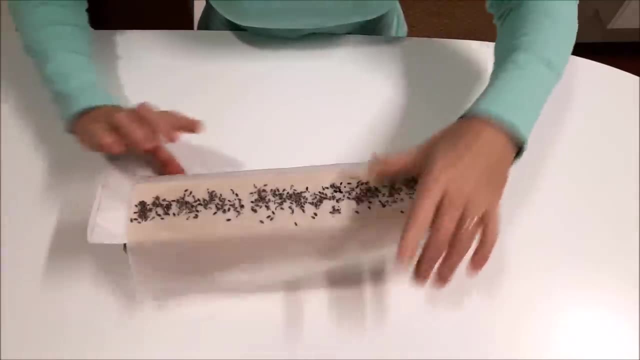 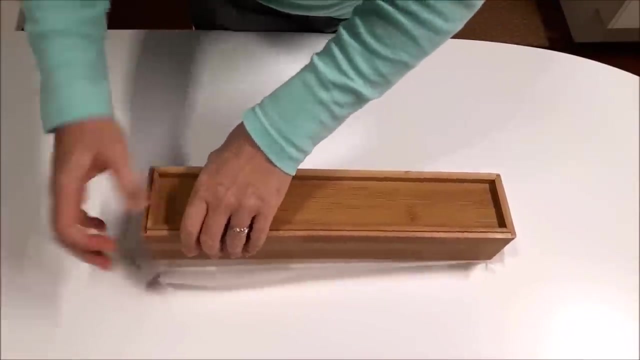 that's okay. it's really purely cosmetic issue, so it doesn't affect the quality of the soap at all. you just get a slightly different, different color. now this can be a bit hard to get out, so I'm going to tip it up and pull it out. that. 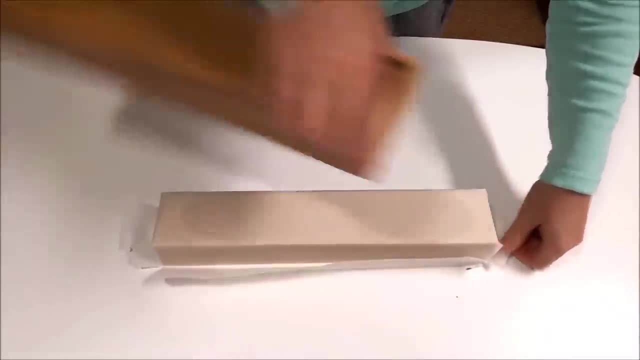 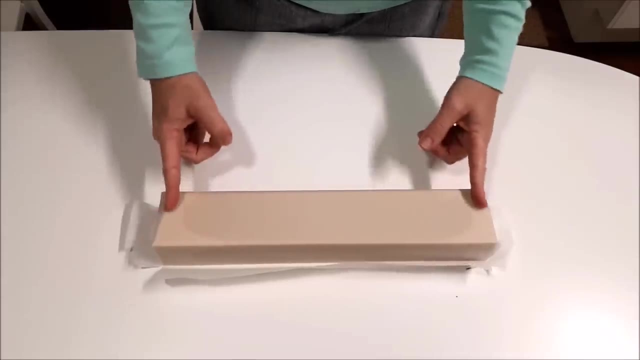 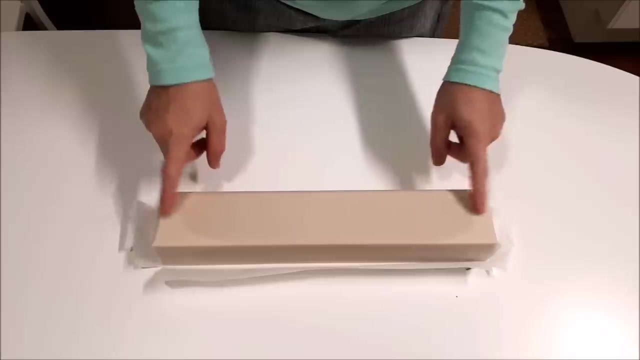 way. oh, it smells so good. oh yeah, wow, so you can see that that line there. that's a partial gel. so I didn't wrap this up enough, so it didn't quite get warm enough to gel all the way to the ends. but that's okay, the soap will be a. 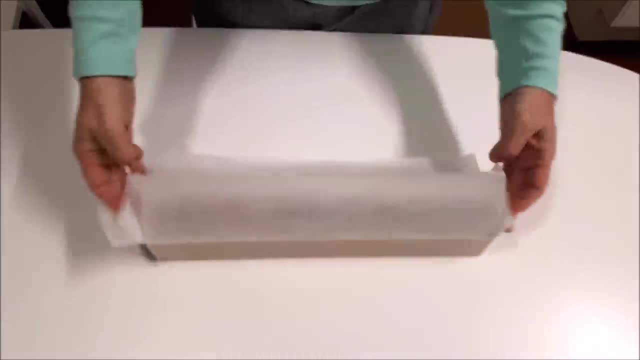 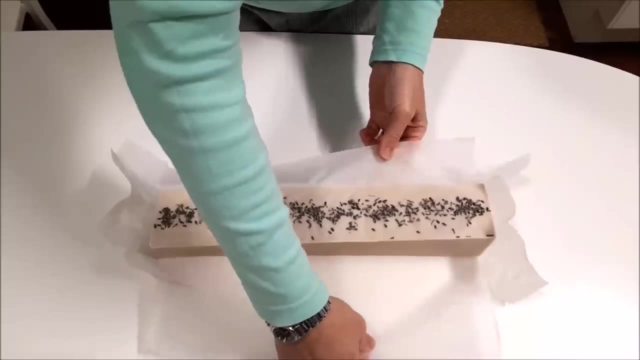 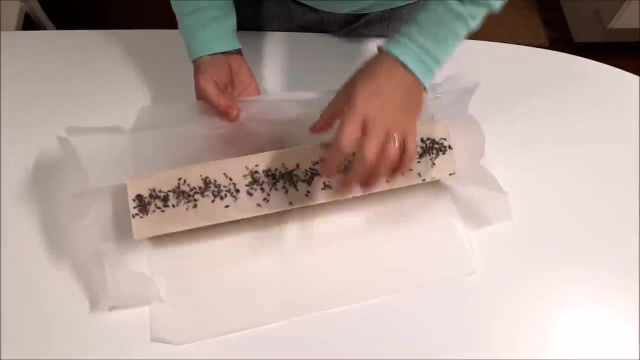 pretty even color anyway, and, like I said, it's it's purely cosmetic. it doesn't make any difference to the soap. I just peel back the paper- oh, this is the most satisfying part- and then I just tip the loaf, oh, over to the side and peel back the bottom bit as well, and then I just leave it on the 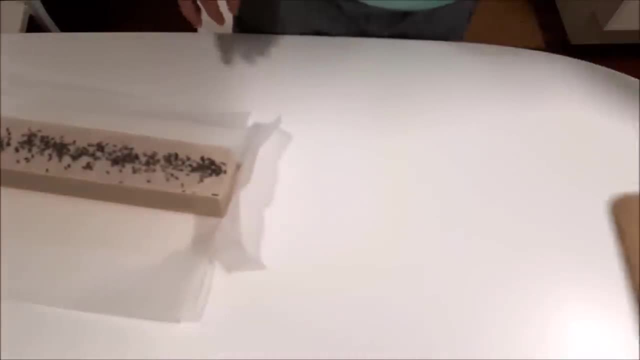 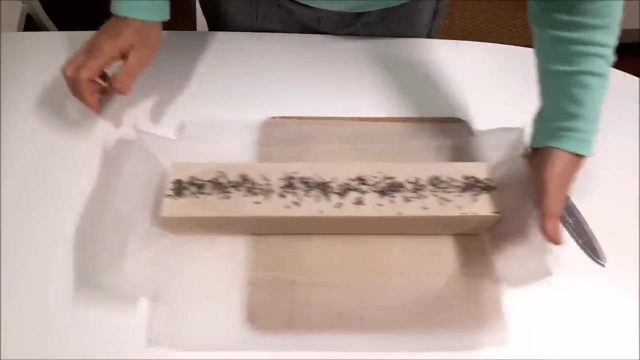 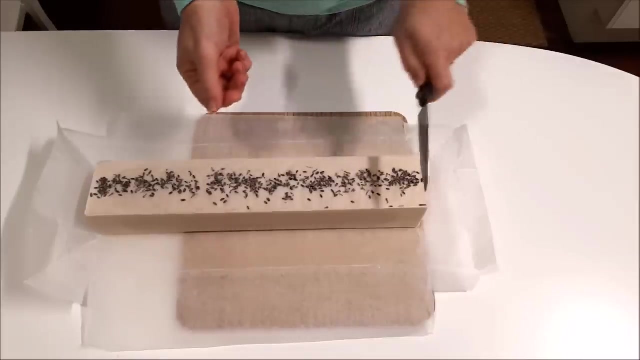 paper. all right, let me get my cutting board. I'm just going to cut this soap just with a knife, which is a very simple way to do it. you can use soap cutters of various sorts, but I find that a good little, just a vegetable knife, as long as it cuts straight. that does the job and I'm going. 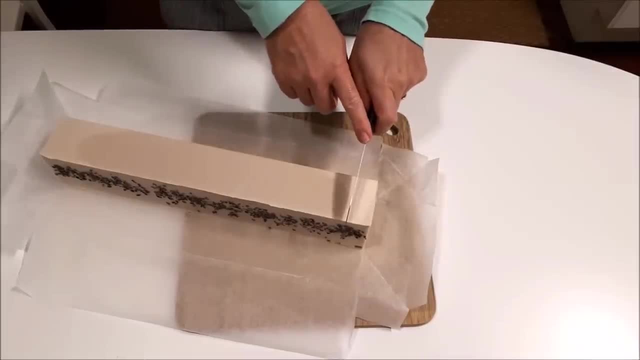 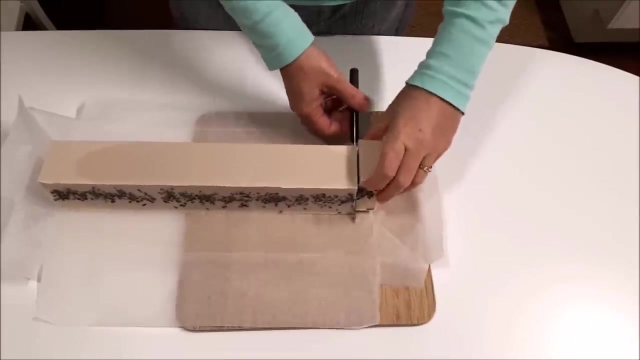 to cut these in roughly sort of hundred gram bars- and I've been, I've made thousands of bars of soap, so I roughly know what that is. try and keep them even in shape. oh perfect. it's perfect consistency for cutting the soap. it does get stuck to the knife a little bit. all right, see that that is our. 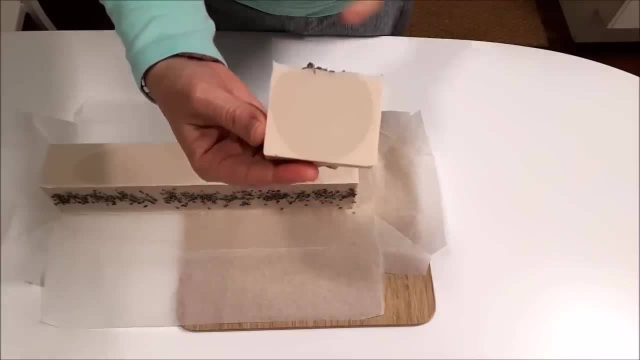 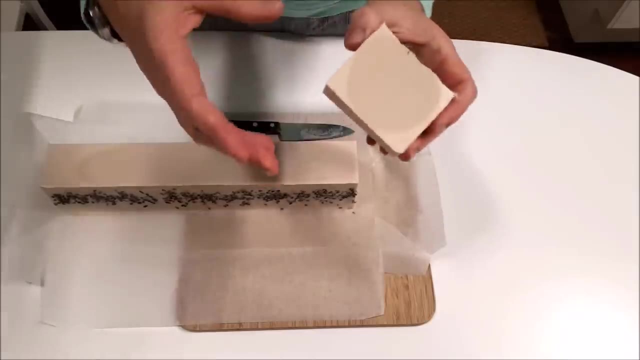 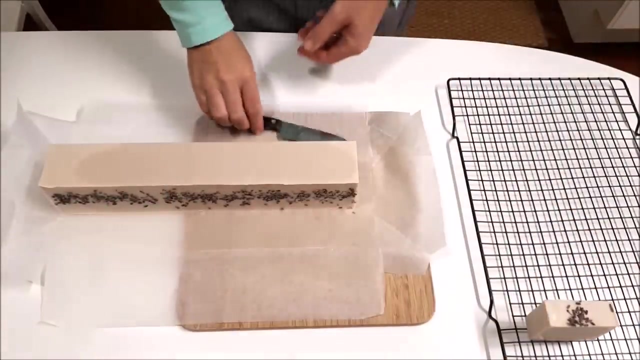 that is exactly what I mean by a partial gel, so the soap is a different color on the inside. it didn't quite gel all the way to the ends, but that's okay. I've got my baking rack here which I'm going to put the soap on, just for now. 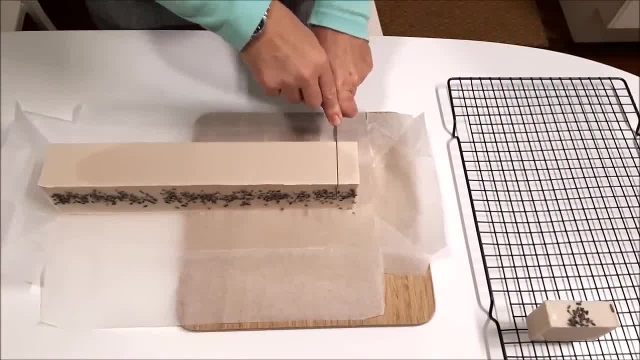 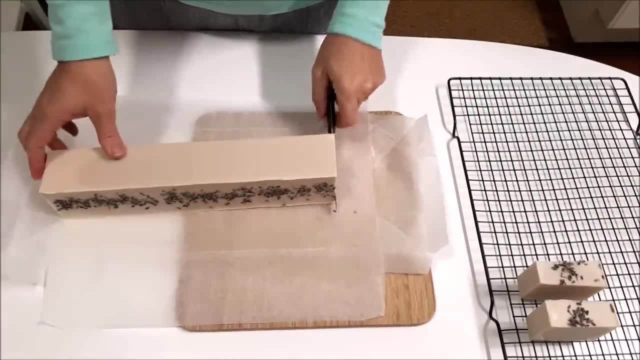 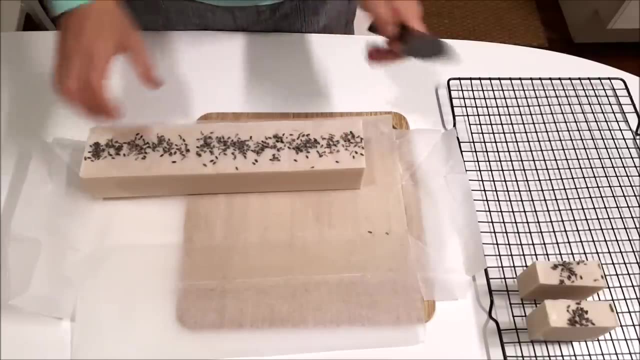 while I cut it. the reason why I'm cutting this on the side is that if I'm cutting it down like that, I would be pushing the lavender buds into the soap, which would sort of wreck the surface of it. so if you've got anything sprinkled, 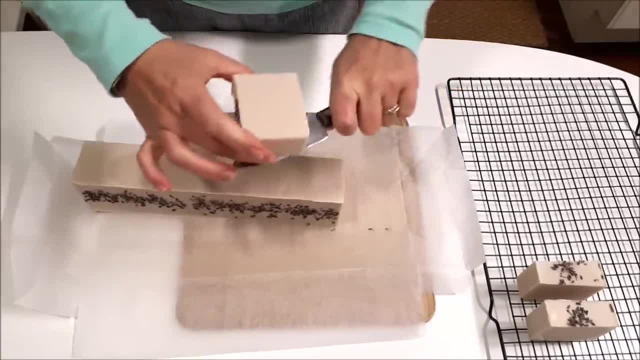 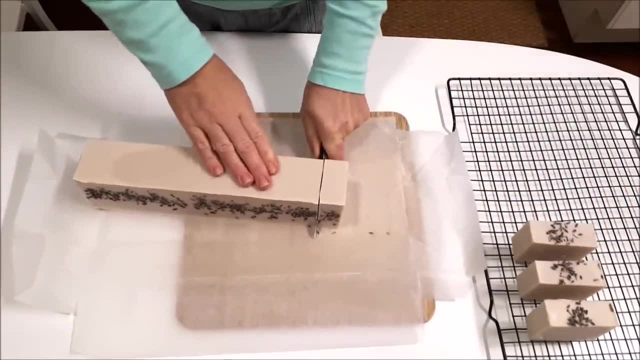 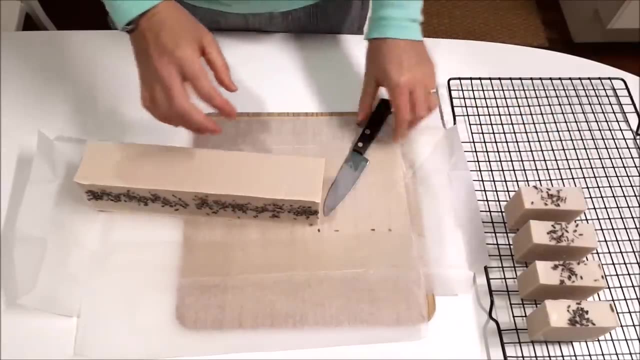 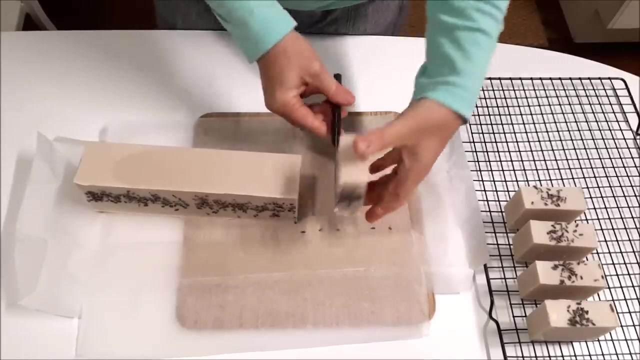 on the top of your soap. just just turn it on the side. oh, that smells amazing. I've got a few friends and family who just can't get enough of the lavender soap, so I thought I'd take this opportunity to make some soap out of the soap. so I'm going to take some. more is the most fabulous smell, if you like. 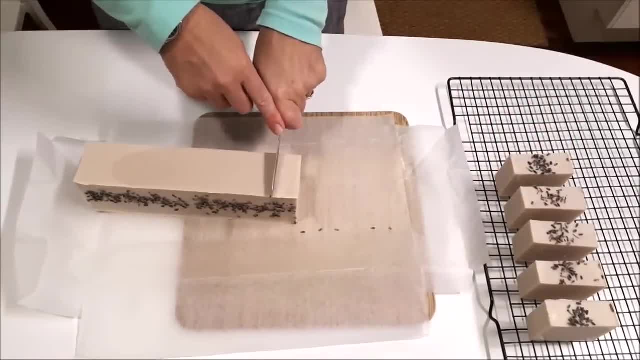 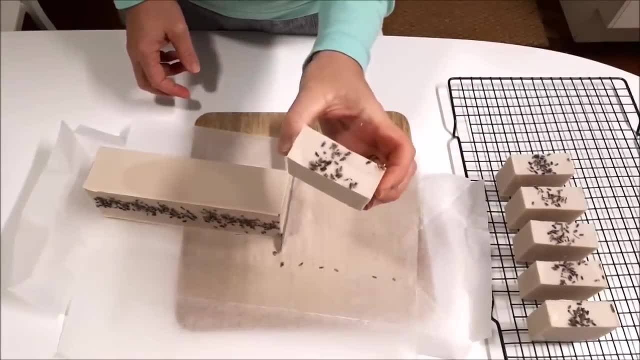 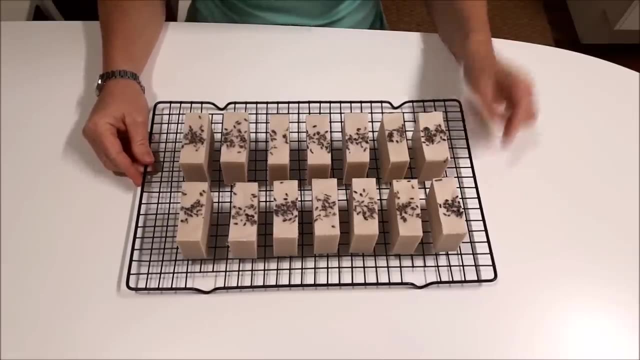 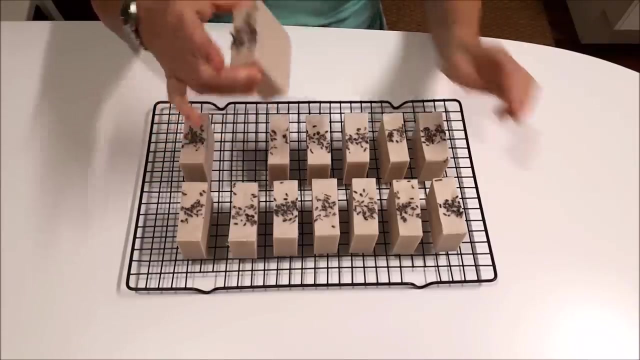 lavender. that is all right. I might just pause this now while I cut the rest of this soap. so there we have it: beautiful lavender, olive and coconut oil soap. I hope you found the video useful and I'll see you in the next video. bye, bye. this soap is still warm. it's giving off the most amazing lavender scent, don't? 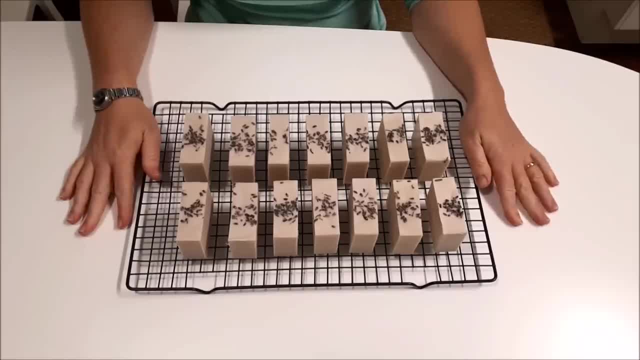 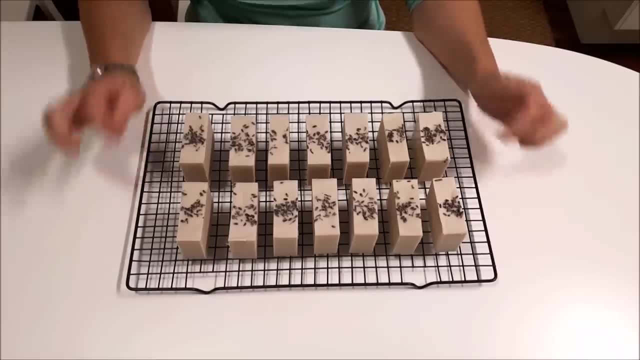 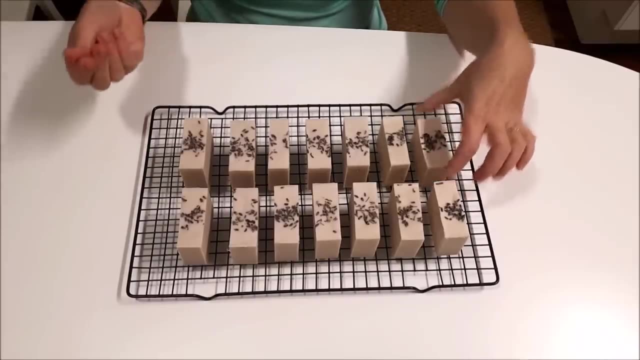 forget that if you just want to make some soap to start with, you don't need the essential oils or the colors or anything like that. you can just follow the basic olive and coconut oil recipe and make make this soap. so what needs to happen now is you'll notice that I was, that I'm just touching this soap with my 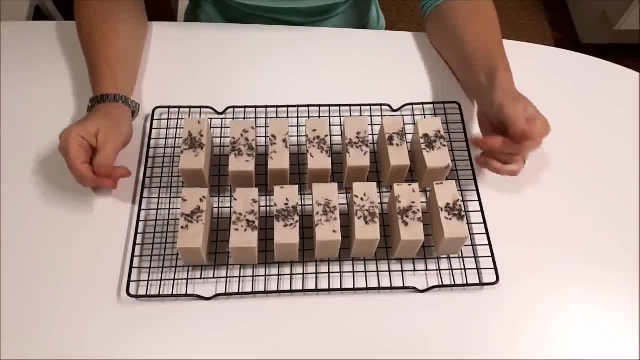 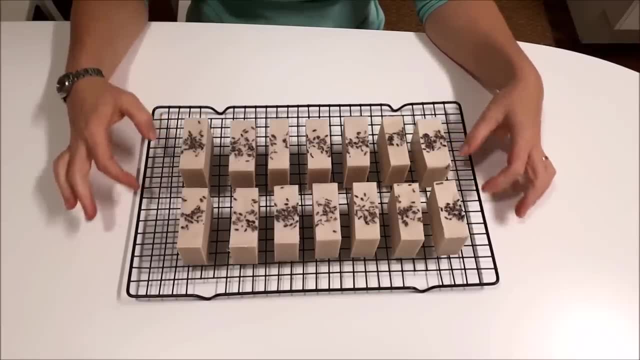 bare hands. it's not completely saponified yet, so it is. it is caustic, but it's not. it's not. it's not completely saponified yet it's not doing any damage to my, to my skin. this will be fully saponified and technically. safe to use within a day or two, but soap generally needs at least four weeks cure time. really, that's a drying time just to make it extra hard and and dry and mild and it'll be ready to go. so store your soap in, you know, on a wire. 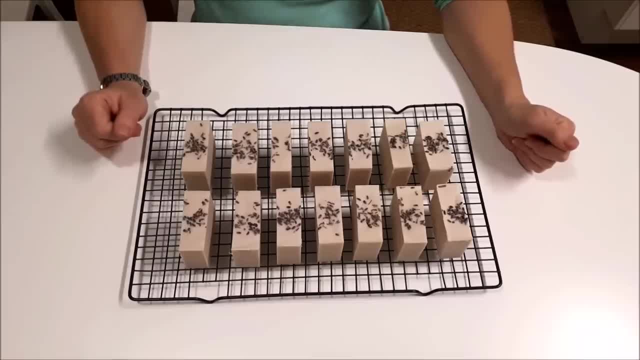 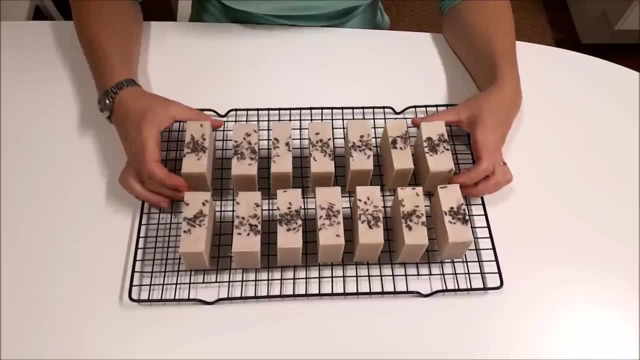 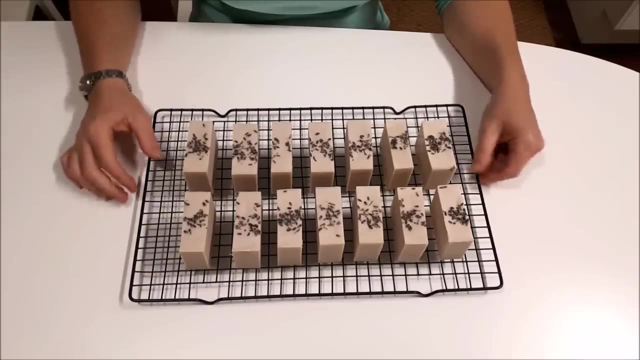 rack like this or some sort of other wire rack and store it in a dry place, if you can. what I tend to do is just while my soap is in the first couple of weeks of drying, I put it down in the laundry because the scent is quite strong and I'm a bit sensitive, so I don't want my even that. smells gorgeous. I don't want my whole house smelling like really strong soap and essential oils, so I put it in the laundry, but then after that I store my soap in drawers, and I just want to show you this quick tip, especially if you live in a humid climate. 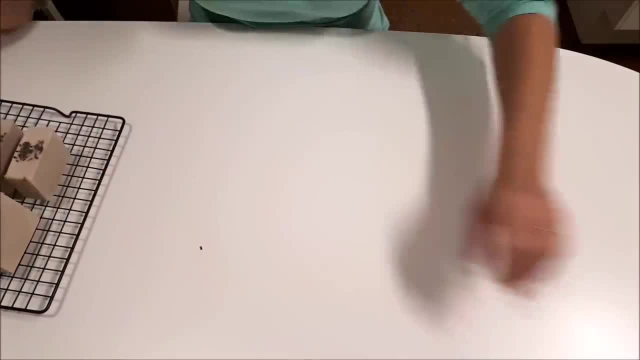 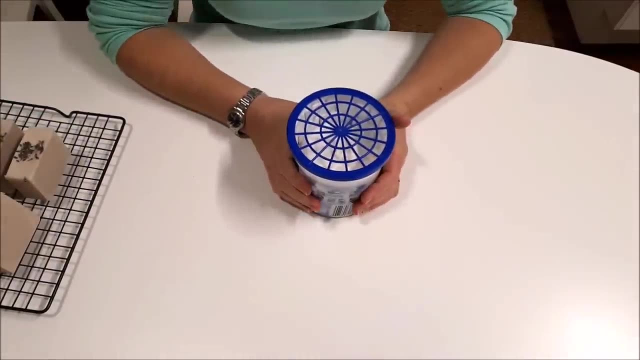 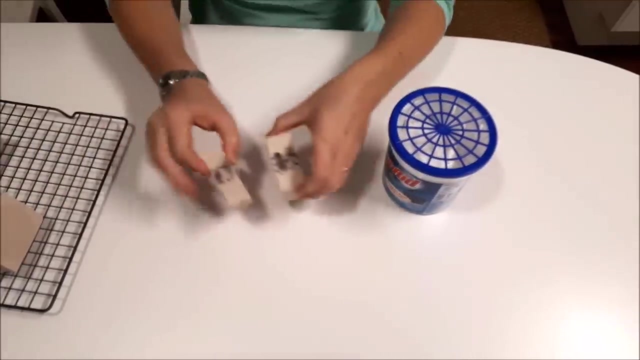 especially if you live in a humid climate like I do. so I have a cupboard in my spare room where I keep all of my soap, and it's just an old cupboard with drawers and shelves. so I put my soap in there and I stack them up, kind of, you know, like that sort of thing in big rows. 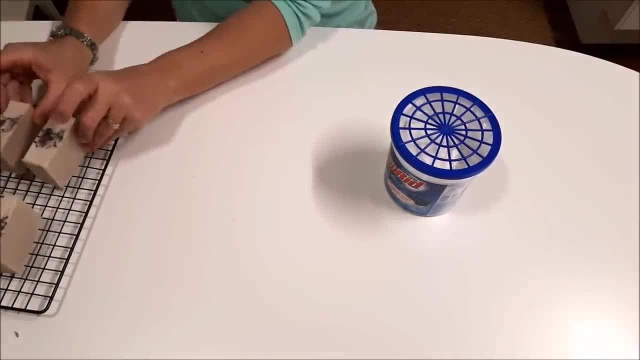 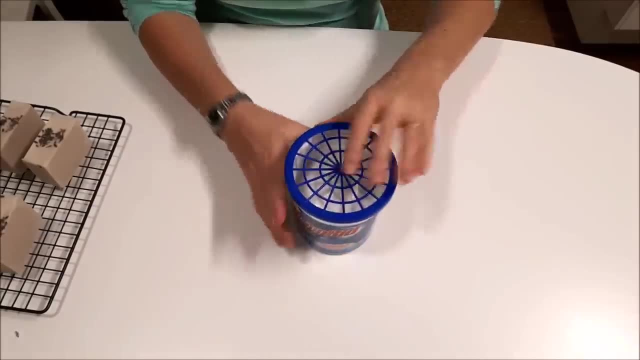 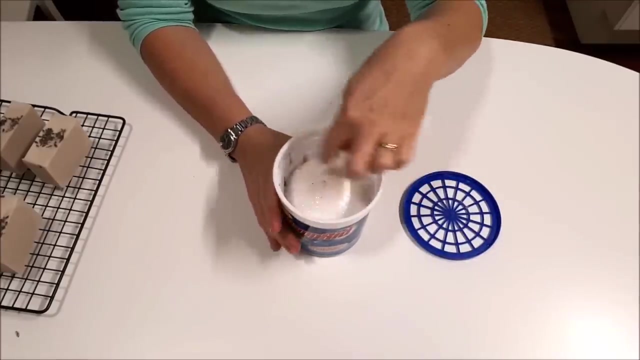 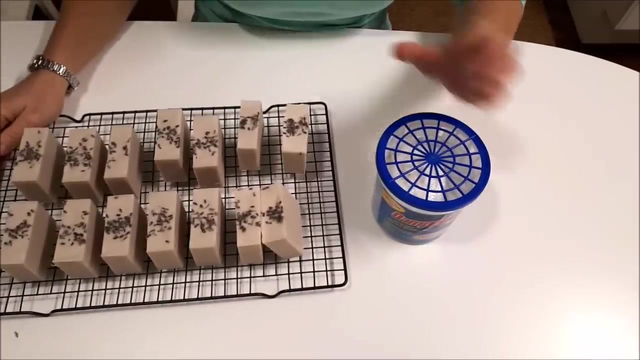 and I. I put one of these things in each drawer and what this is is a dehumidifier, so you can buy this from the supermarket or the hardware, and they're refillable, and what they do is this. I think it's calcium carbonate. it attracts moisture, so you could put your soap in a storage container or some other. 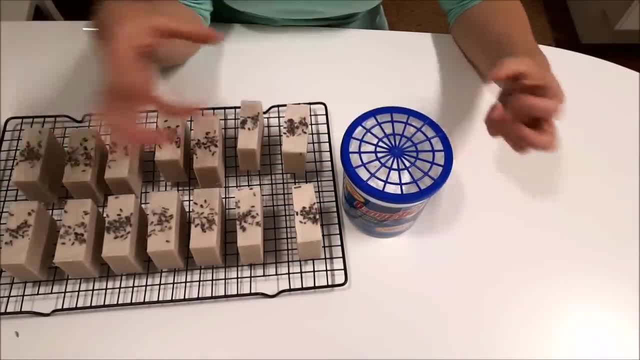 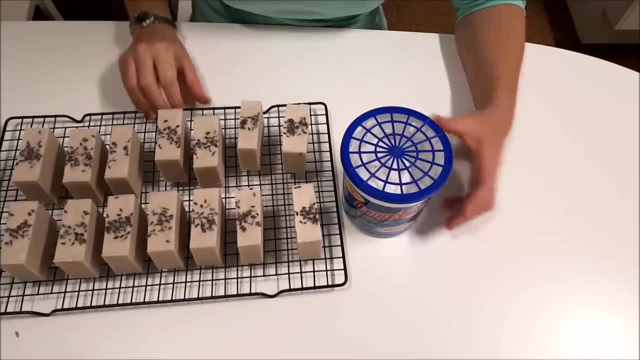 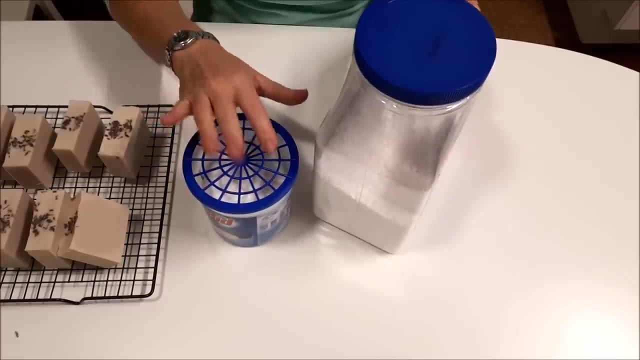 sort of closed in drawer or something with one of these, and it will continue to draw moisture out of the air. so your soap will keep drying while it's um, while it's covered up. and you can buy these big refill containers of this stuff. There's various brands that you can get. 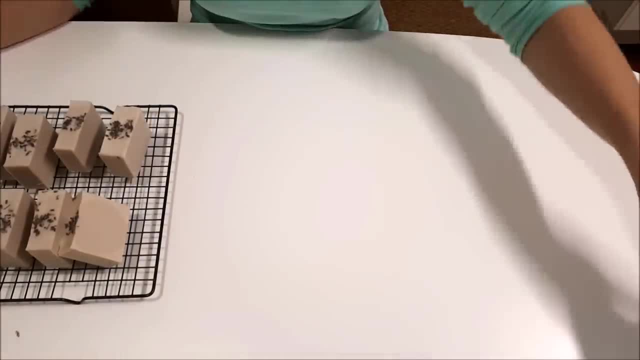 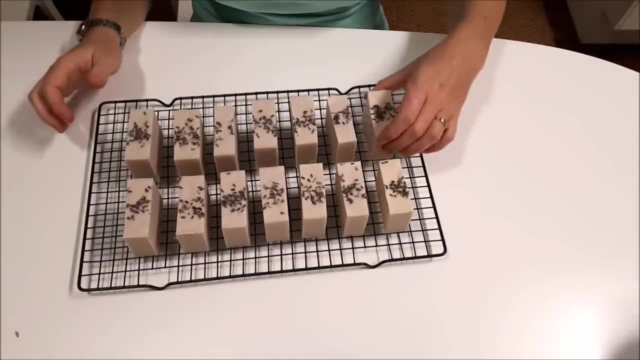 I like this brand. it's easy to use, So that's a great way to store your soap, particularly in very humid weather. Because soap is a salt. it is hygroscopic, which means it attracts moisture. So in very humid weather, your soap. 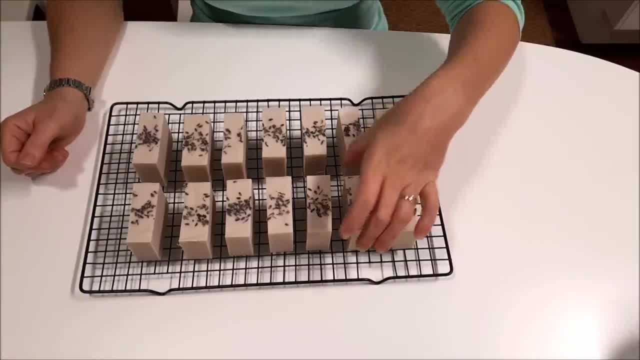 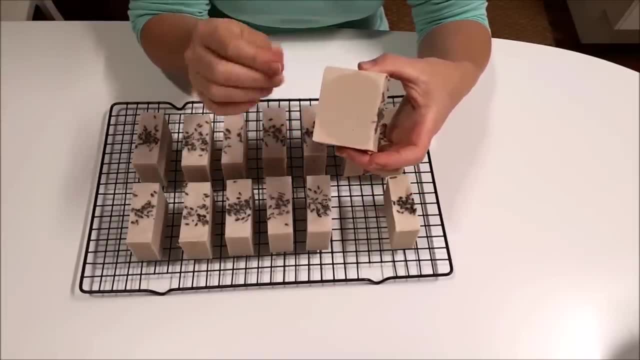 it won't dry very well. it will take a really long time And sometimes you know if it's raining outside and you've got all of your windows open in high humidity, you'll actually feel a slimy dampness on the surface.